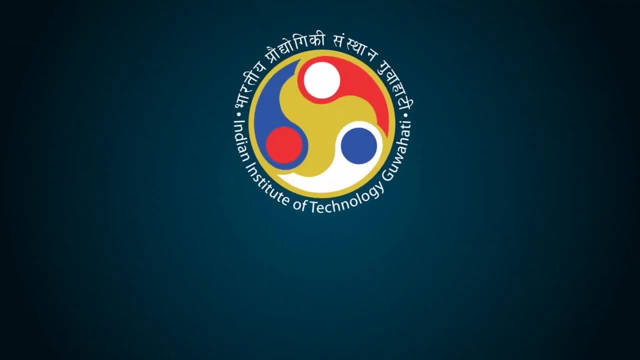 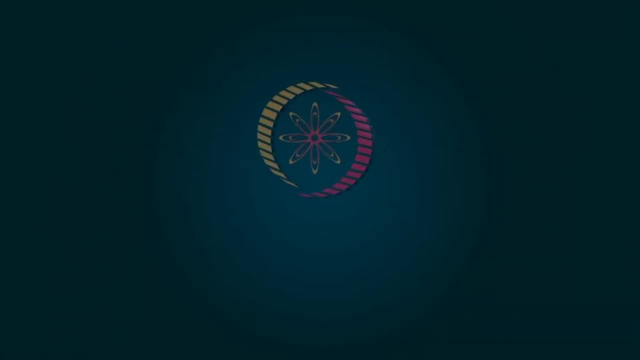 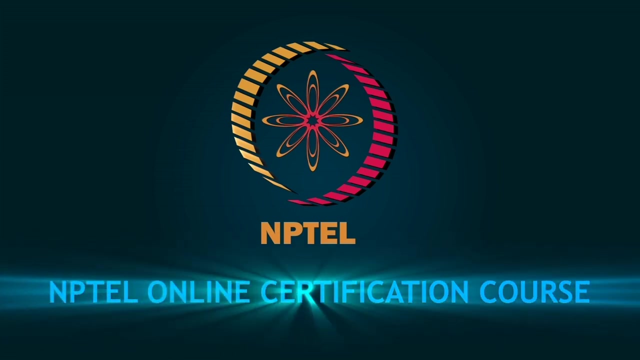 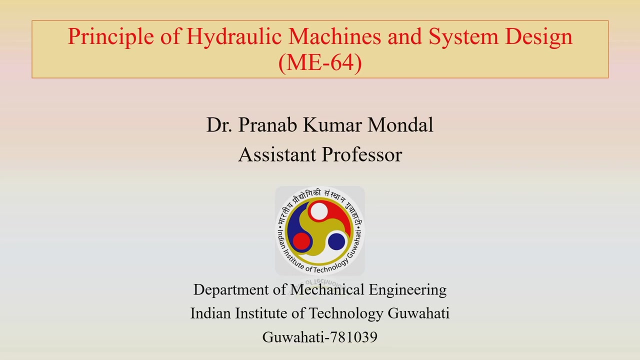 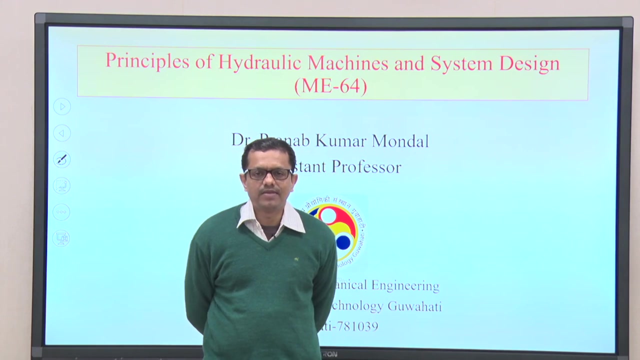 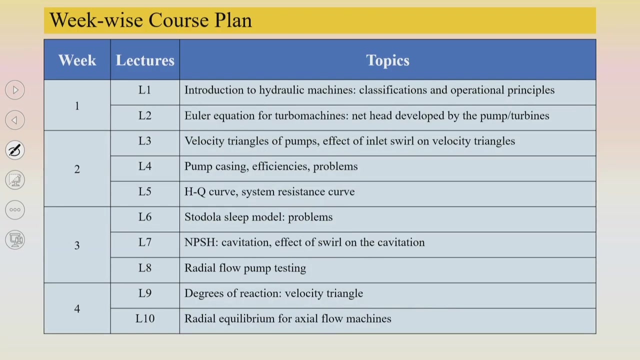 Thank you for watching. Good morning. I welcome you all to the session of principle of hydraulic machines and system design. In this course we will discuss different modules of the hydraulic machines, So I would like to show first lecture wise, different modules that will be covered in this course. 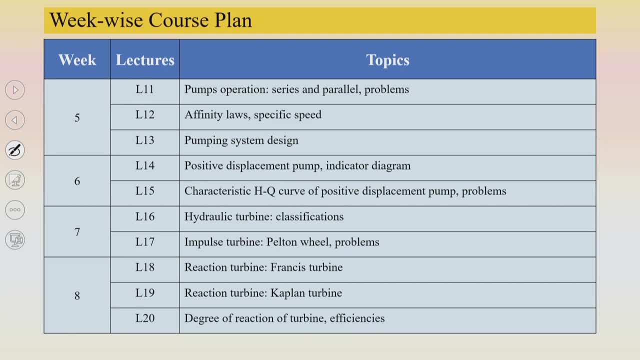 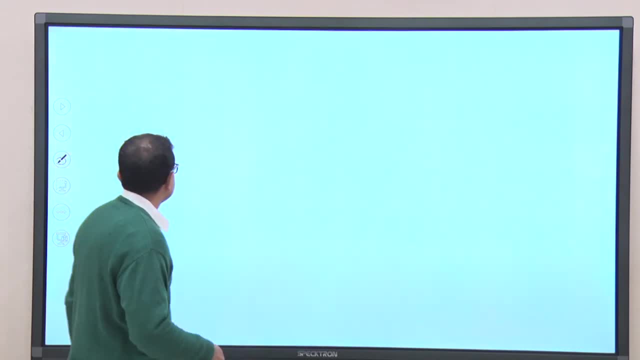 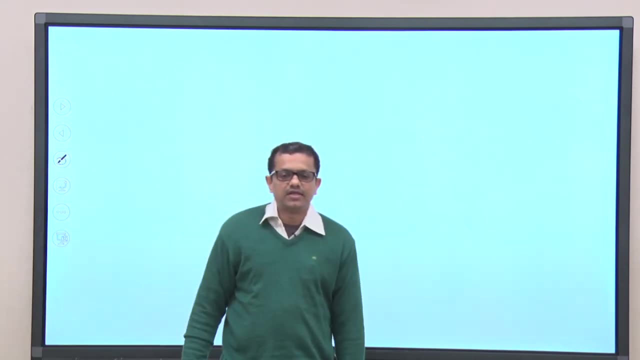 and then we will move to the next module. We will discuss the topic which I will. I have this I have decided to discuss today. So if we now try to discuss, if we try to find out different aspects of hydraulic machines, We have studied fluid mechanics and we have seen that these hydraulic machines, which is 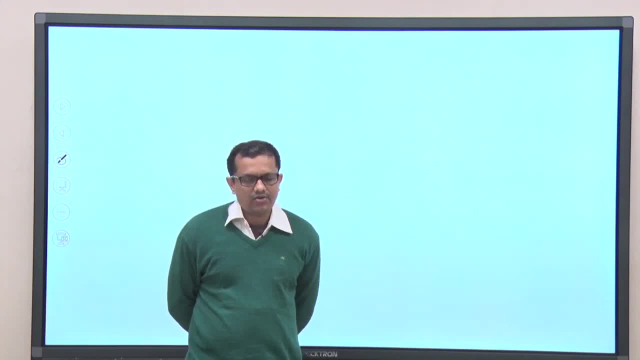 a special class of fluid machines, of course, which are used for the conversion of energy, either from mechanical energy to the fluid- I mean stored energy of the fluid, or vice versa. Before I go to discuss the classification of fluid machines, which is the topic of today's discussion, I would like to tell you that 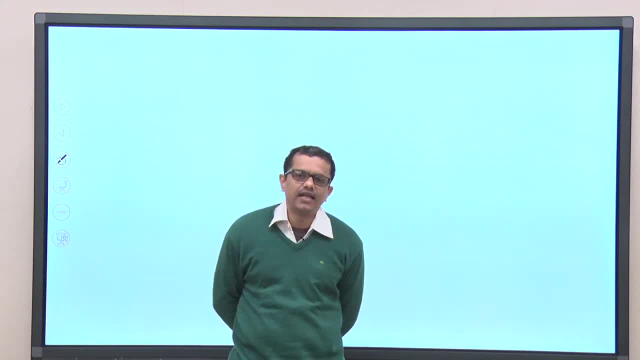 ah, We have encountered different types of fluid machines in our daily life. right In this room, in this class room, there are fluid machines. What are those? Like fan blower. We also, you know, see in our daily life that pump is used to supply liquid from the ground. 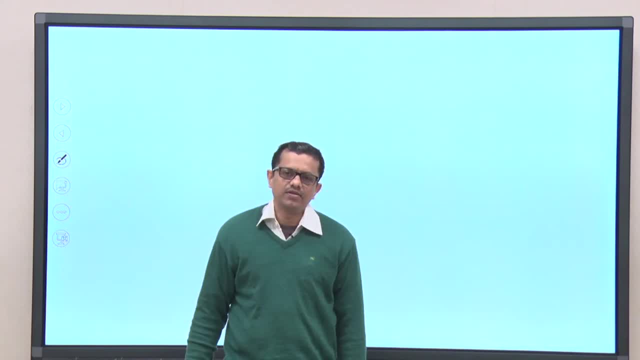 water tank To the tank which is situated at the top of the multi-storied building. So, for the example that I have given, there are also- you will find examples, that- which are used to supply, you know, liquid, rather fluid, from one place to other place. 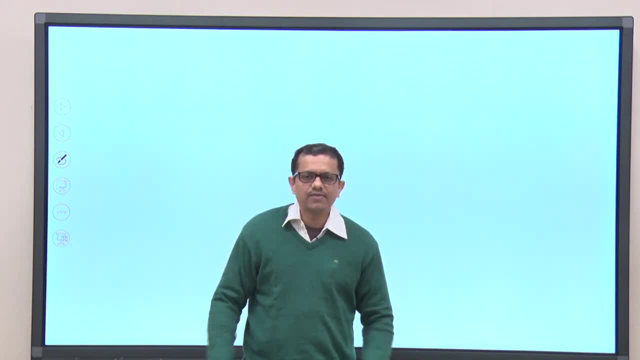 What we can see from this, you know, what we can understand from these examples, is that there are fluid machines, There are fluid machines, There are fluid machines And these fluid machines, they are operating. their operational process, their operating principle is basically different And in all these machines there is a working fluid, rather 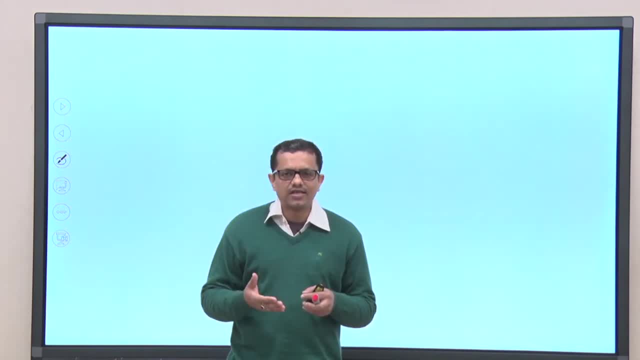 the working medium of the energy conversion. that is what I was talking about, that in this fluid machines energy is getting converted from mechanical to the stored energy. So the energy conversion of the fluid is converted to the stored energy of the fluid or vice versa. 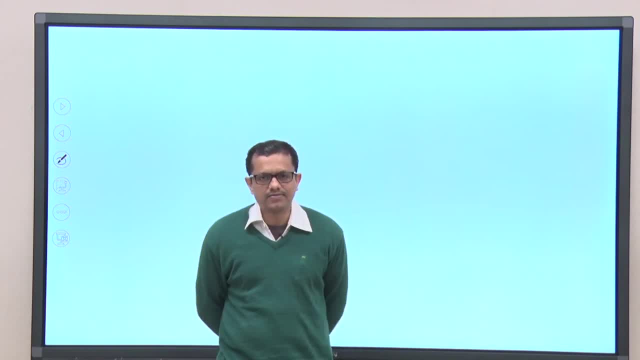 That is, from the stored energy of the fluid into the mechanical energy. Whatever may be the case, in all these cases they are. I mean we need to have one working medium, That is, a working fluid. So, based on the types of working fluid and also the direction of 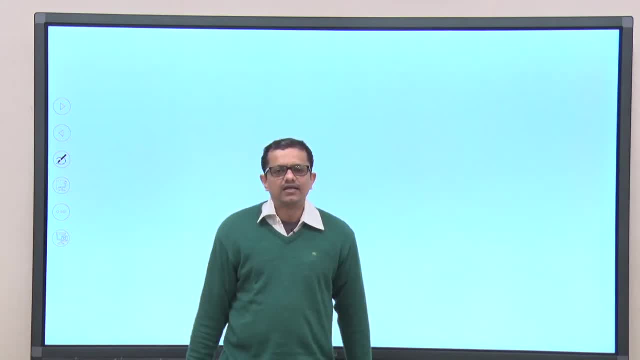 energy conversion conversion and, finally, depending on the direction of fluid, because, as I said, that we need to have working fluid, working medium for the energy conversion. So there will be a direction of fluid flow, because it is not the case that fluid will fluid will be static in inside. 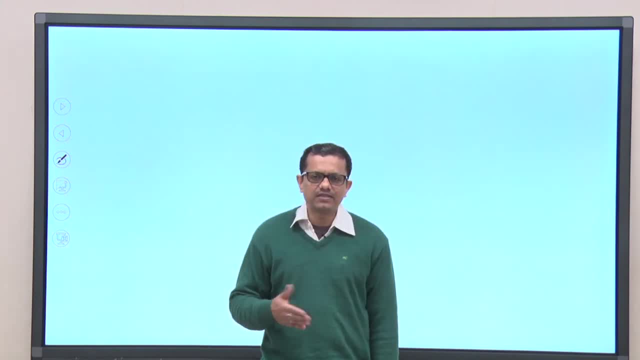 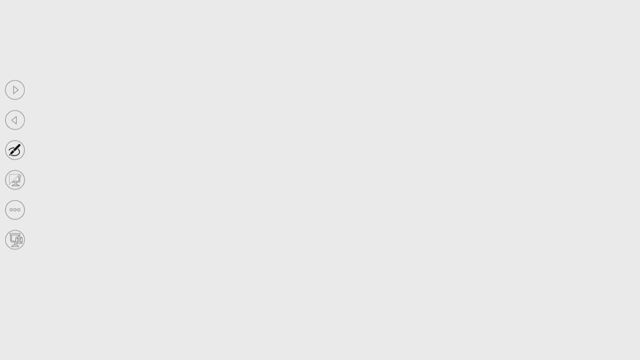 the machine right. So depending on the direction of fluid flow inside the machine, we can classify fluid machines into different categories. So now I am going to write classification of, you know, fluid machines. 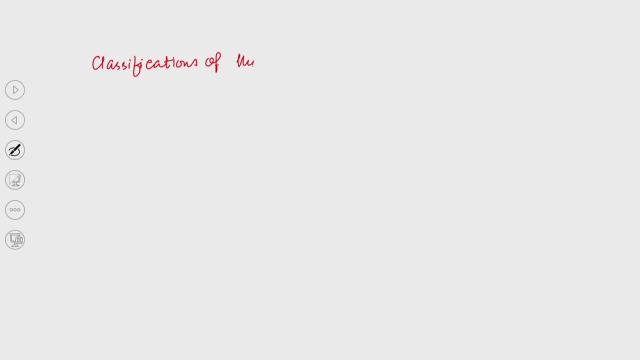 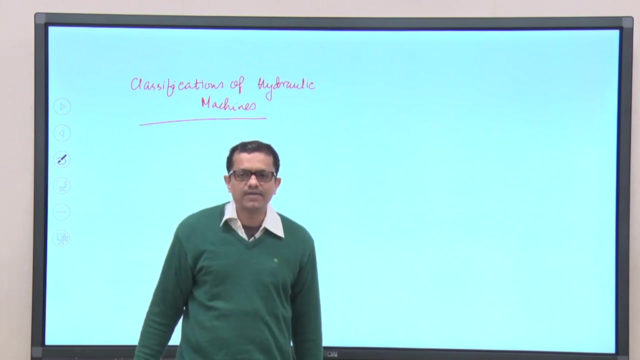 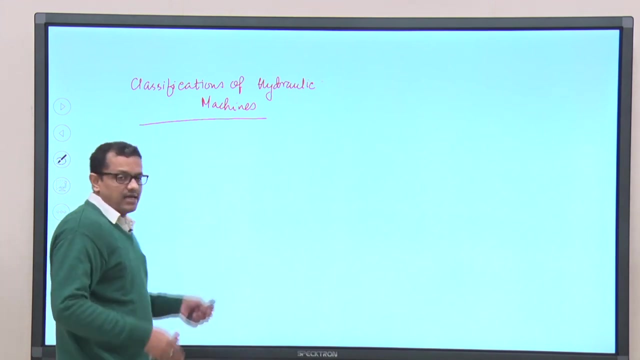 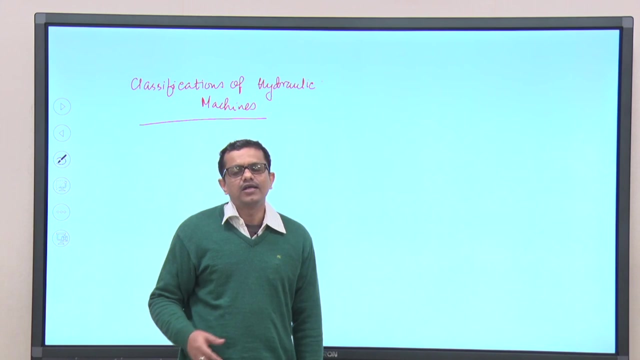 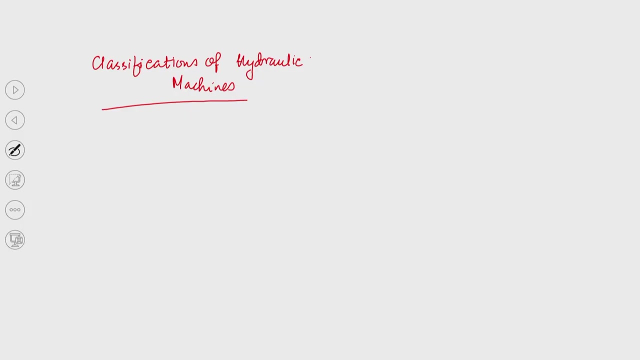 crouch for shelter liquid water. So if we try to classify, this can be classified into two different main. 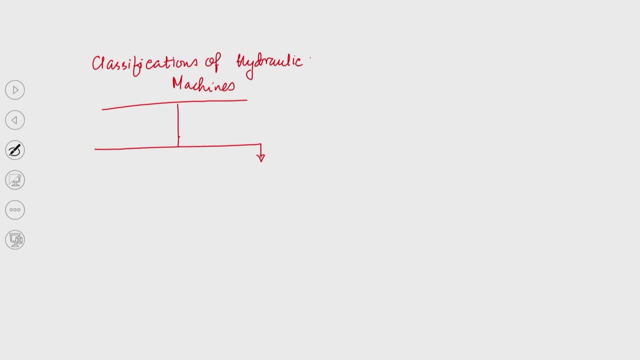 groups. one group is pumps and other group is turbine. So this is the main group and this is turbines, this is hydraulic turbine. So pumps and turbines. I have written hydraulic turbine because turbine we know we have. we have studied that steam turbine is there. 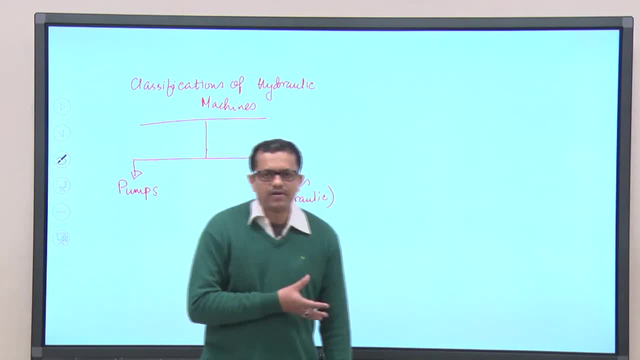 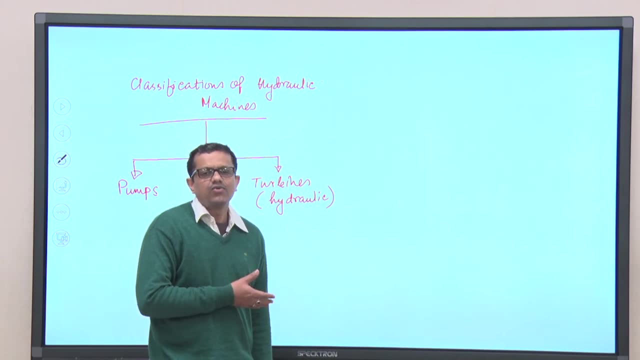 gas turbine is there In all examples, whether it is steam turbine, gas turbine or hydraulic turbine. So we can see that there is a working fluid which is used to exchange energy, whether from stored energy of the fluid into the mechanical energy in case of the turbine. But in today's 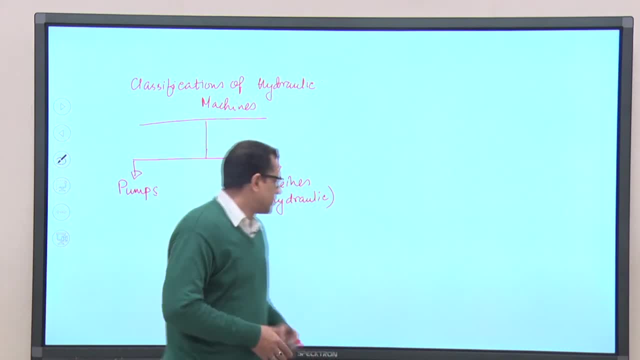 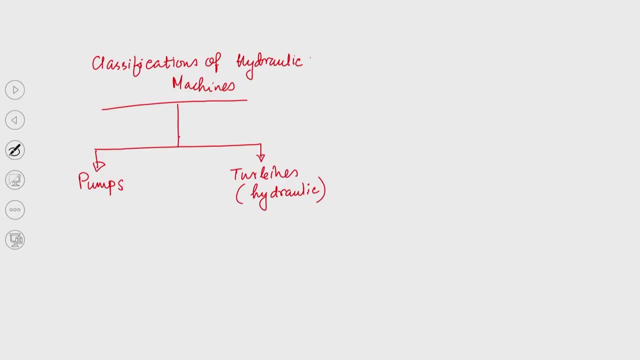 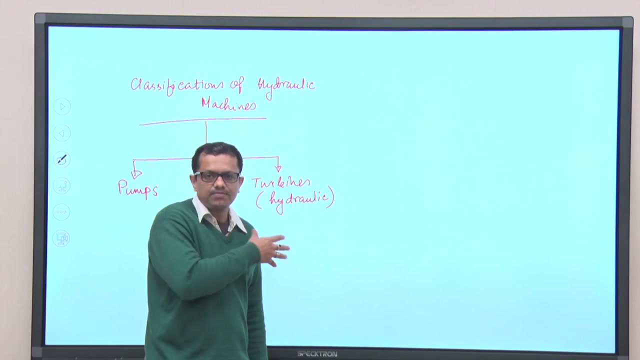 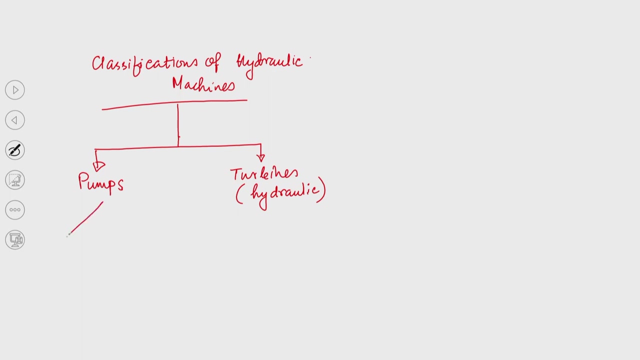 I mean in this particular course we will be focusing on the hydraulic turbine. The pumps can be, again you know, sub classified the you know pumps and turbines. we will discuss turbines later again the details because this part is there in this course. This pumps can be sub classified into three different. I can say you know two different groups, one: 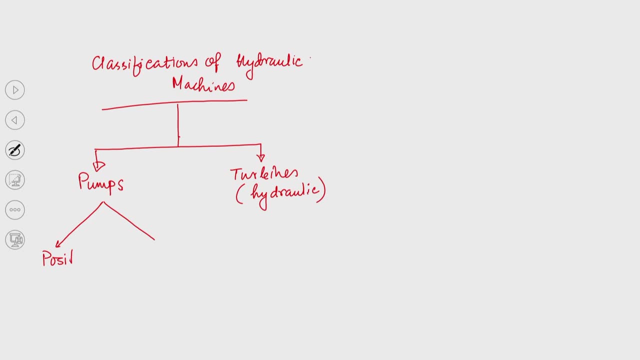 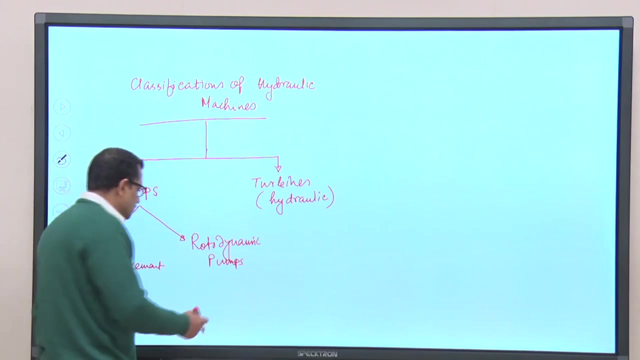 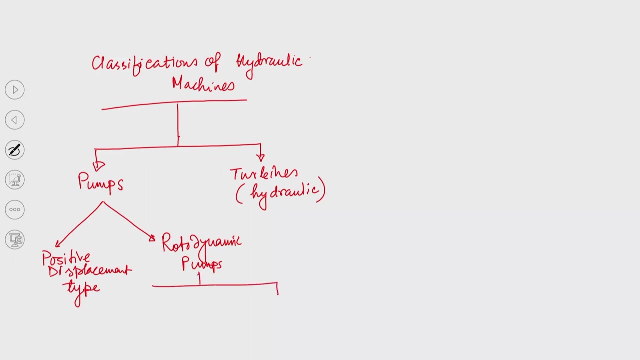 is known as positive displacement type. second one is known as rotodynamic rotodynamic pumps. So this rotodynamic pump again can be classified into three different categories. I am writing here this is: one is radial flow. second one is radial flow. second one is radial. 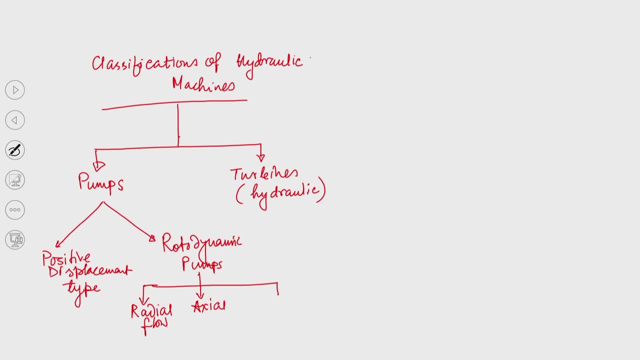 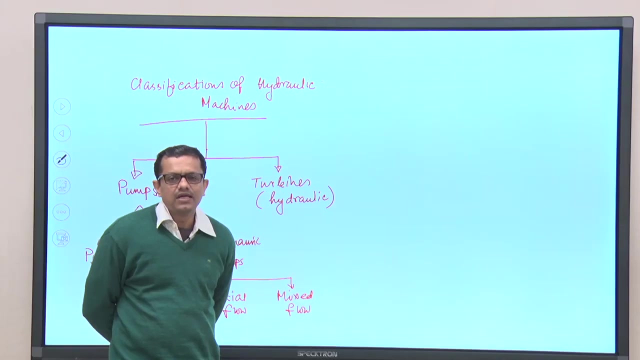 flow: Axial flow. third one is mixed flow, right, So this pumps we can classify into two different categories. one is positive, displacement type. second one is Rotodynamic. pumps can be further subclassified into three categories: radial flow, axial. 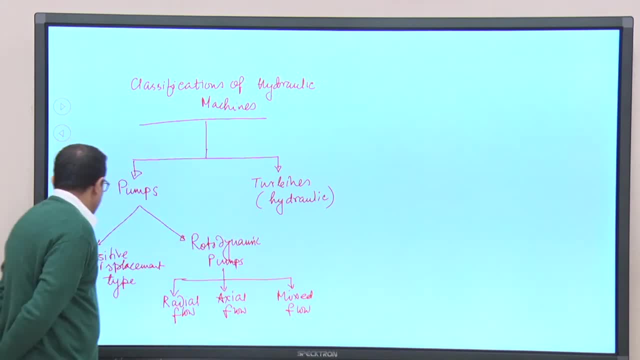 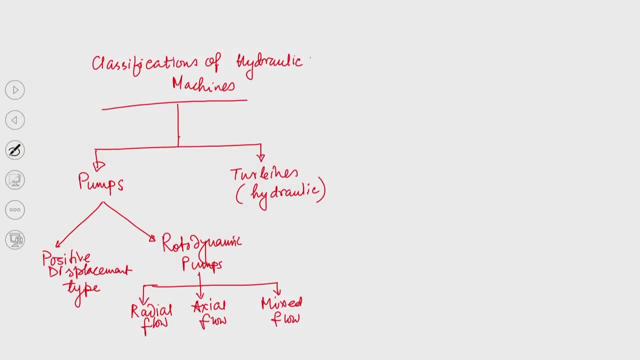 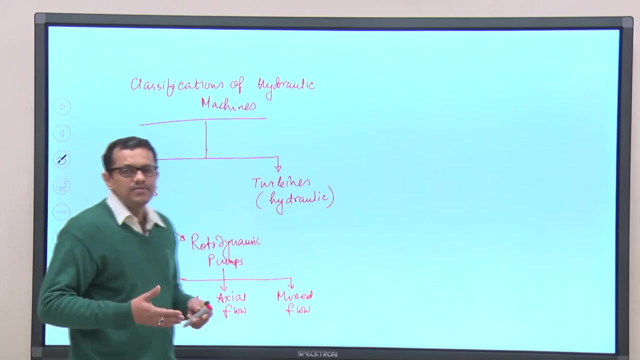 flow and mixed flow. right, And I will discuss later now, when we are trying to classify pumps into two different subcategories, that is, positive displacement type and the rotodynamic pumps, What is the basis of this classification? At least we should know at this point of time. okay, 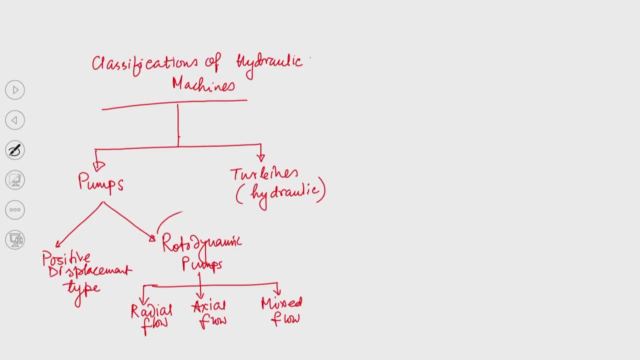 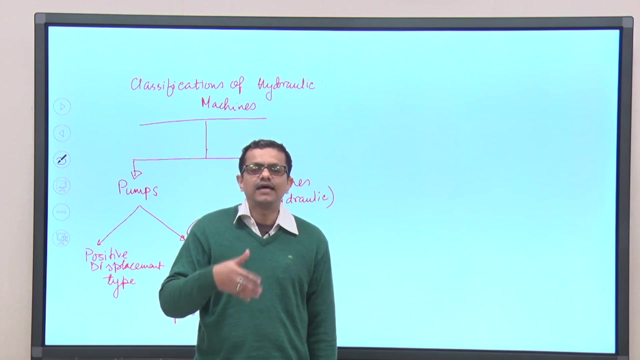 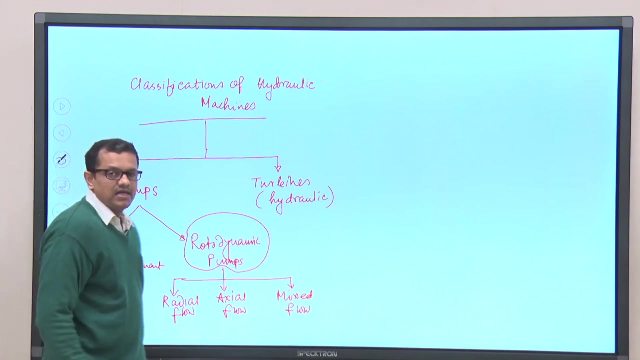 So you know this rotodynamic pump we can see from the name itself rotodynamic. so there will be one rotating element, rotor, and it will have dynamic action: rotodynamic pump. Then, for the positive displacement pump, there is no such, you know, rotation I mean. 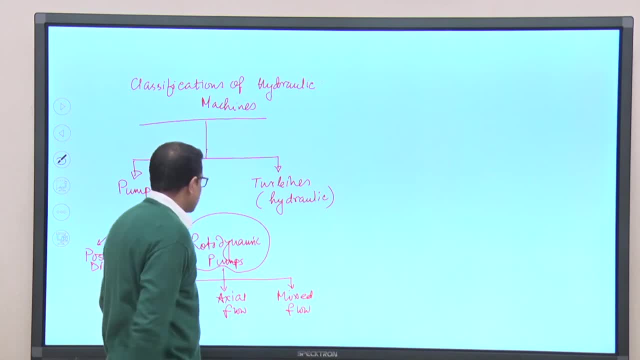 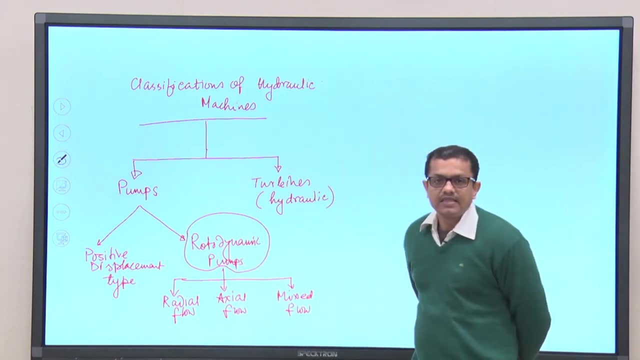 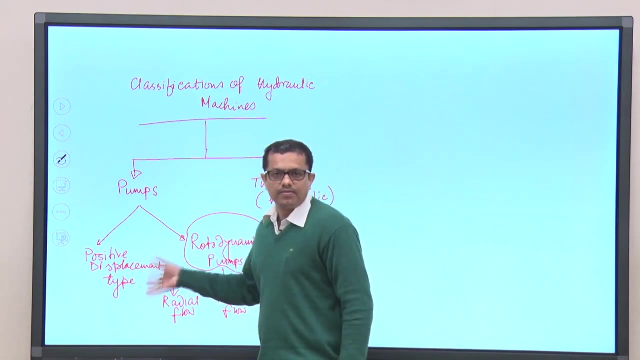 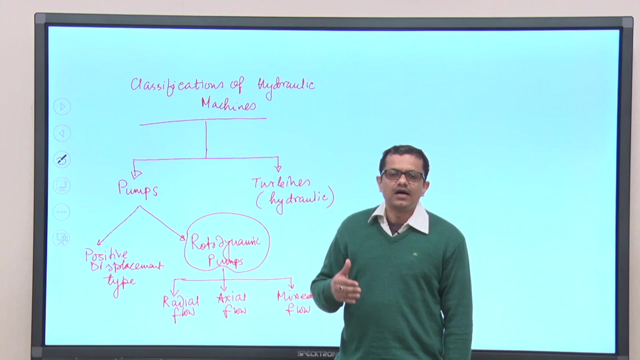 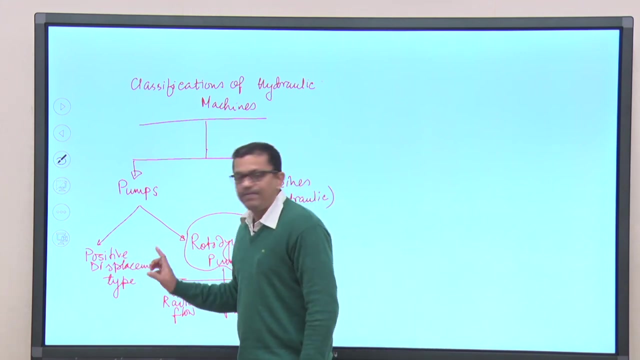 rotationality effect. right In this context, I will tell you that the positive displacement type, this positive displacement pump, the functioning of this group of pumps, is essentially based on the fact that there is a change in volume of certain fluid mass, And the word positive displacement is coming from the fact that the certain amount of fluid 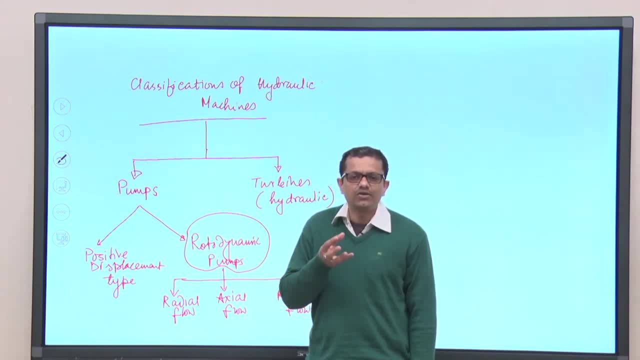 mass. if we consider this mass as a control mass system, there will be a physical displacement of the boundary of this control mass. So that is why the name positive displacement type is coming. So two things First. one is First of all positive displacement, that means the positive displacement pump, the functioning 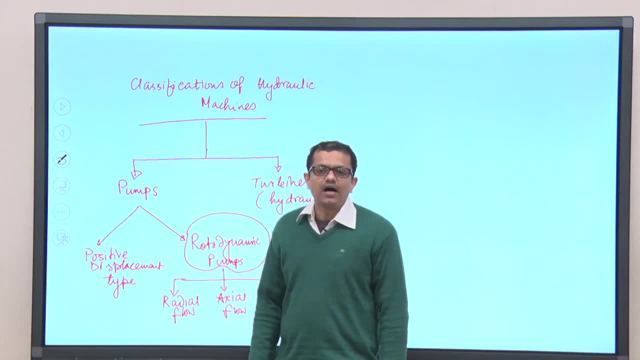 of this type of pumps are based on the fact that there will be a change in volume of certain fluid mass and the certain fluid mass if we consider as the control mass system, there will be a physical displacement of the boundary of this control mass. 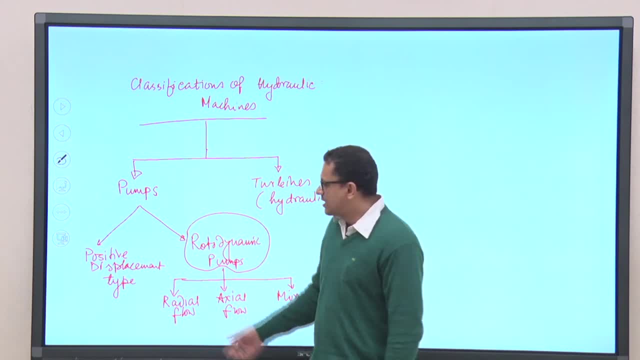 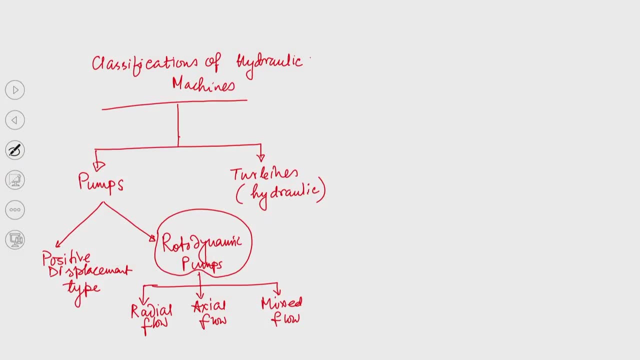 So that is why positive displacement is the word. positive displacement is coming. This pump can be further. I mean, there are different types of positive displacement pump. I am just writing over here: positive displacement pump. Okay, Okay, Okay, Okay. 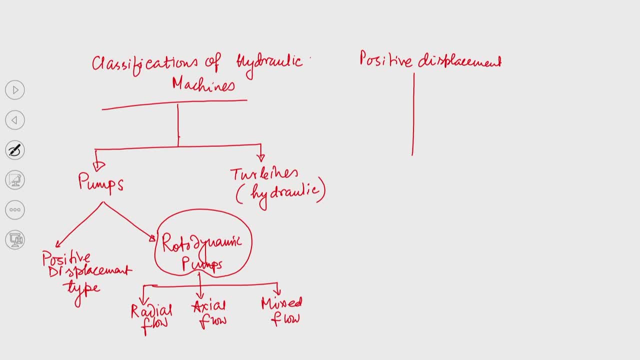 Right. you will find in different text books screw pump, gear pump, van pump, reciprocating pump. this at theingen formation is implemented in different text books. So that is why negative displacement pump has higher fin zrobing parameters. 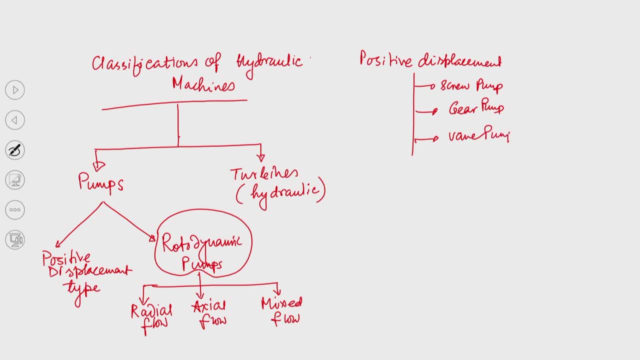 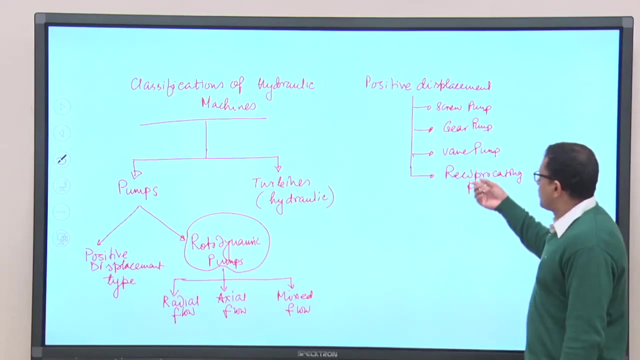 Okay, So this is that is why positive displacement of the boundary of this control mass is. this type of pump has higher fin zrobing parameters. Okay, So this is what this is- the form of a positive displacement. We have seen positive displacement pump. we have seen that we very often we need to go. 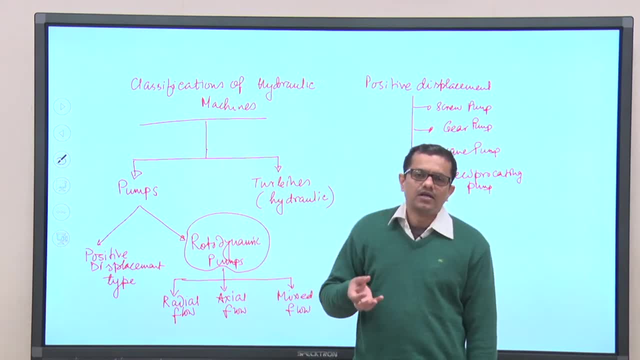 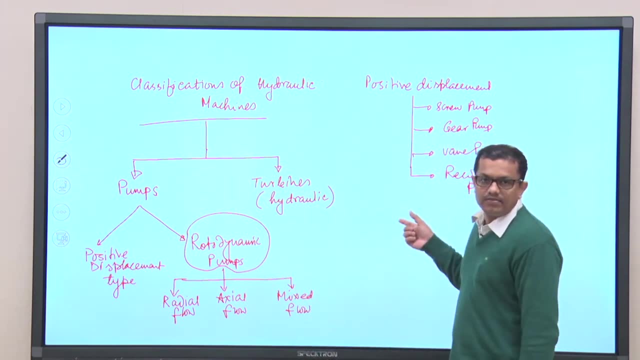 to cycles of for, rather to supply air into the wheel, and this is done using reciprocating pump and that is the positive displacement pump. So we consider certain fluid mass as a control mass system and there will be positive displacement of the boundary of the control mass in the process. while we are coming to rotodynamic, 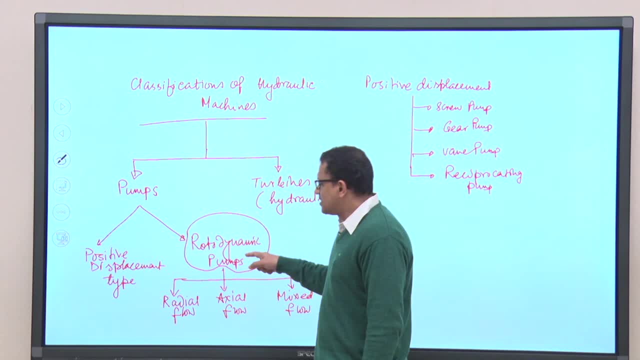 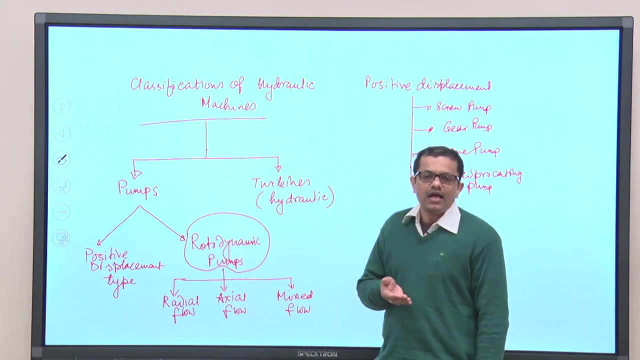 pump. as I said you, that means the working principle of the pump, rather of the of the of these pumps, depends on the rotationality of the pump. Rotationality effect- I mean rotational of the mechanical elements, rotor, dynamic rotor at that- that means there will be a rotating element and by virtue of rotationality effect, 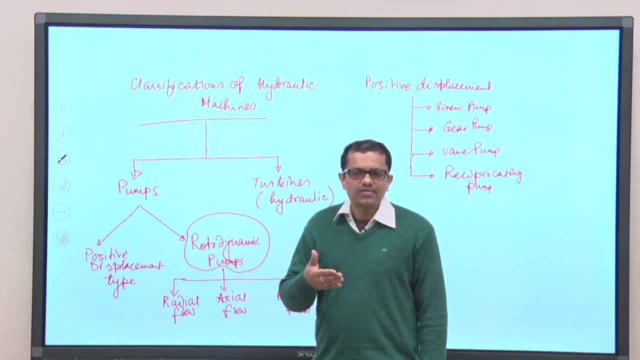 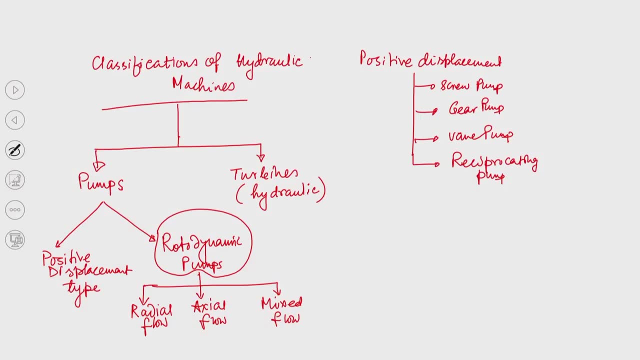 there will be a transfer of energy, fluid, dynamically. So I am now telling this turbine, hydraulic machines and rotodynamic pumps. sometimes these are known as Turbomachines. I will tell you later, but for the time being, at least we should know. 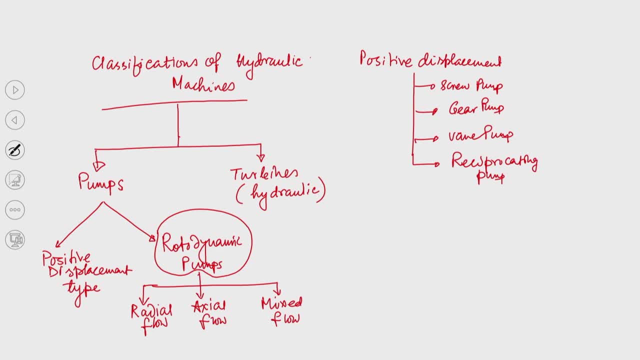 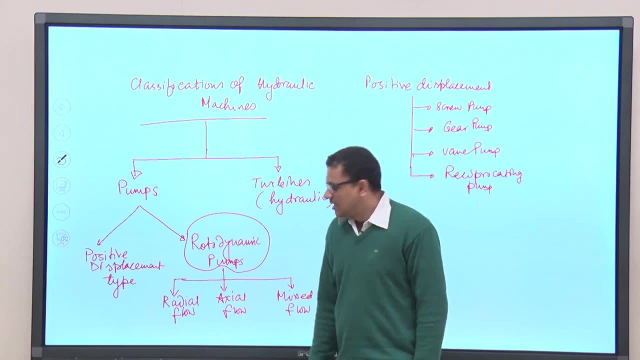 here this: rotodynamic pumps can be classified into three different groups: radial flow, axial flow and mixed flow. so that means you can see from, you can see from this classification- radial flow, mixed flow and axial flow. so that means we are having this classification. 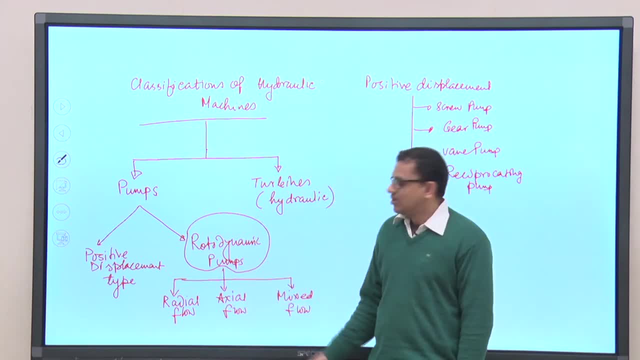 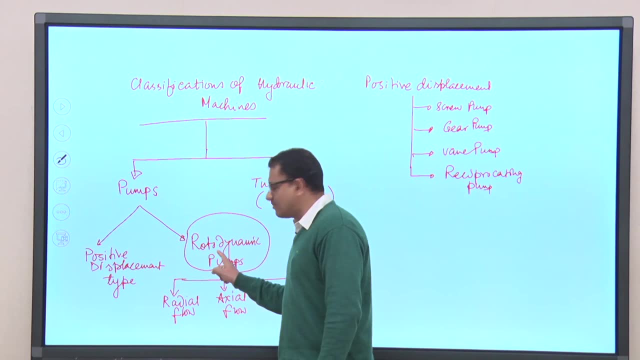 based on the direction of flow. So this classification is based on the direction of fluid flow, while positive displacement pump and rotodynamic pump, this classification is based on the mechanism of energy transfer inside the pumping pump. And finally, I would like to tell you the rotodynamic pump and turbines. these are sometimes 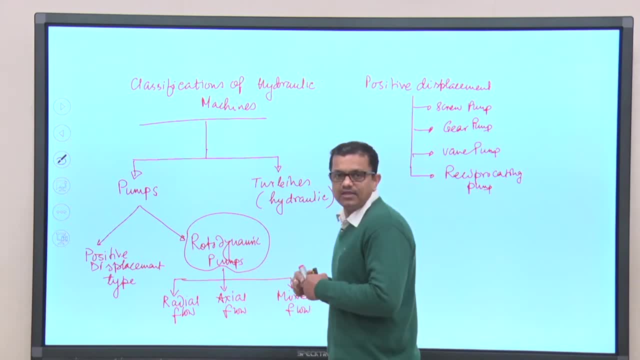 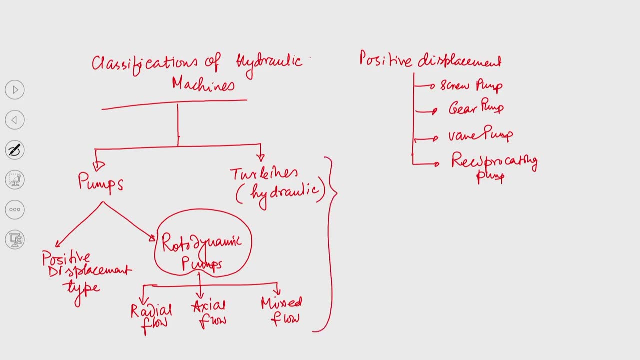 are very often known as turbomachines. so I will briefly touch upon this aspect again. So this you know: turbines and this rotodynamic pump, this are this type of- I mean these machines are sometimes known as turbomachines. 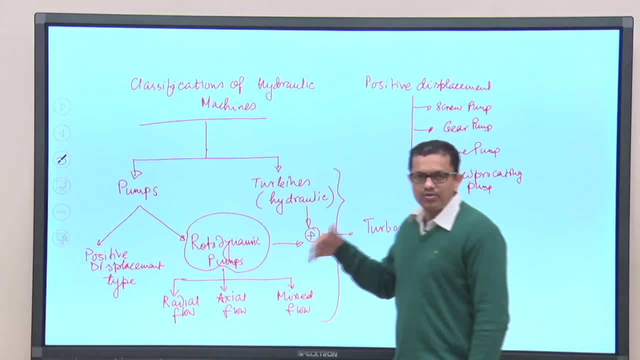 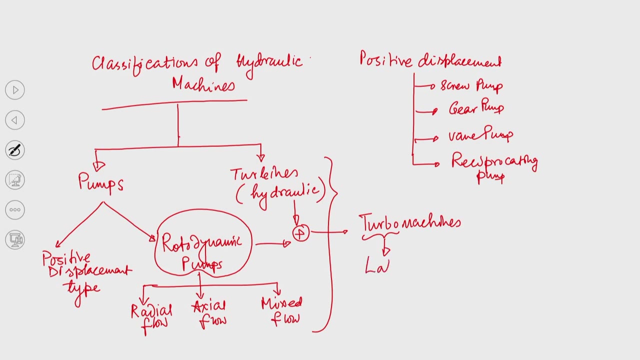 So, since today I am focusing more on, you know, mostly on the classification, so I am thinking that I should discuss this aspect here. Turbomachines: the word turbo is coming from one Latin word, Turbinis. 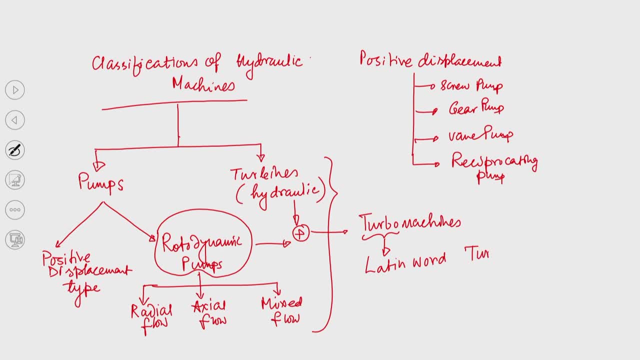 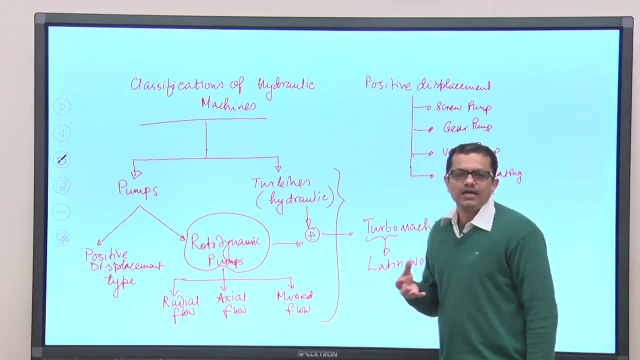 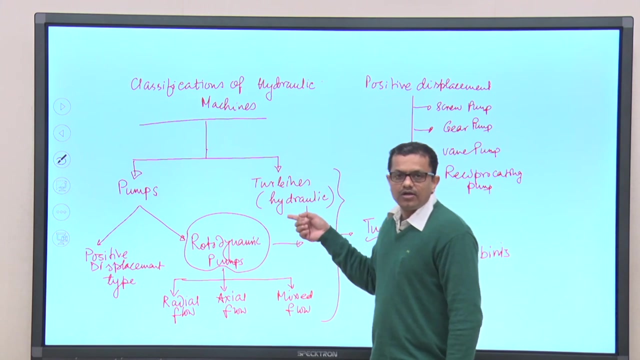 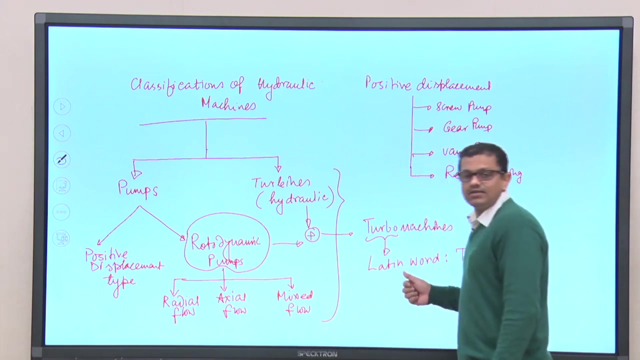 The word turbo is coming from a Latin word, turbinis. what is the meaning of turbinis? Whirling, swirling motion, that means the working principle of these group of machines, turbines and roto-dynamic pumps- depends on the swirling action. rotationality effect, whirling motion. 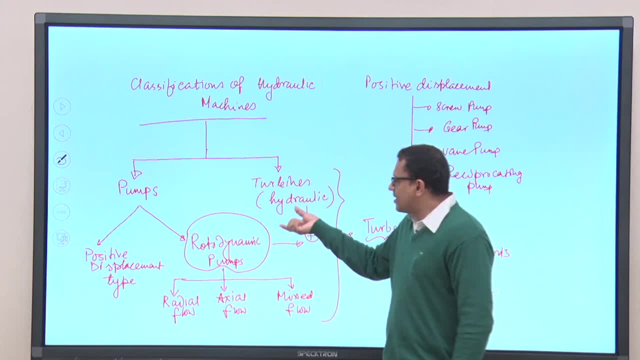 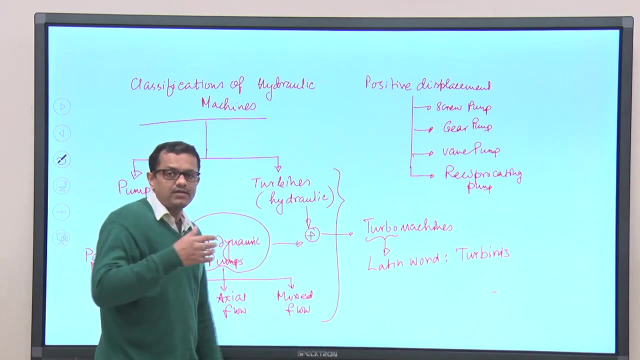 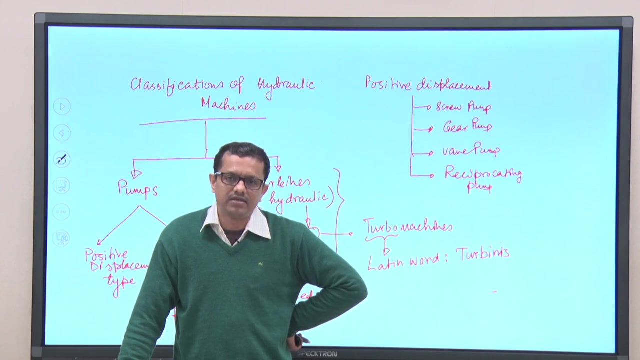 So that is why these are, rather these machines can be grouped together and they can be said as the turbo machines. fine, Now we have seen that hydraulic machines working fluid is water, and this can be classified into two groups: pumps and turbines. what we can see: 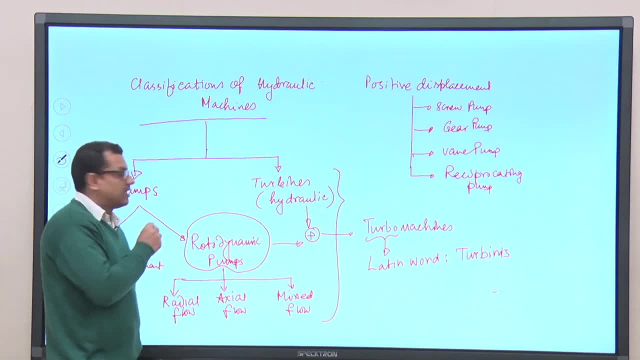 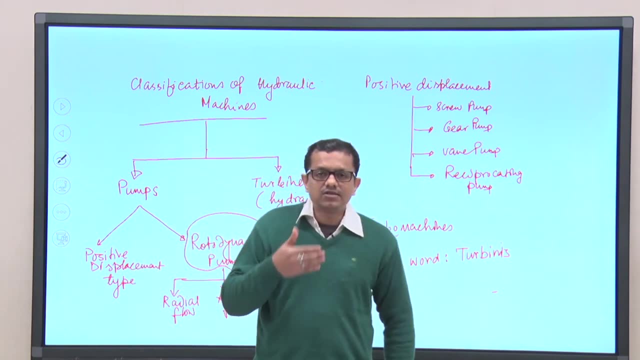 So the first classification is based on the fact that, In pumps, what do we do Using pump? we install pump to supply water from ground water tank to the tank which is situated at the top of the building, in a multistoried building, of course. 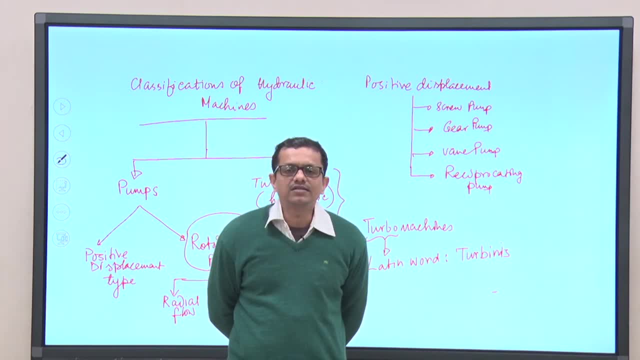 So what do we do using pump? We need to increase head, we need to increase pressure. we will discuss this aspect again in our subsequent lecture. So basically, what do we do? we increase pressure using the pump. So if we now look into this- the working principle of pump- from the aspect of energy conversion, 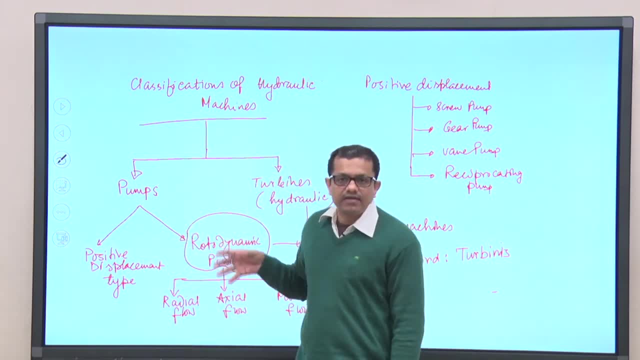 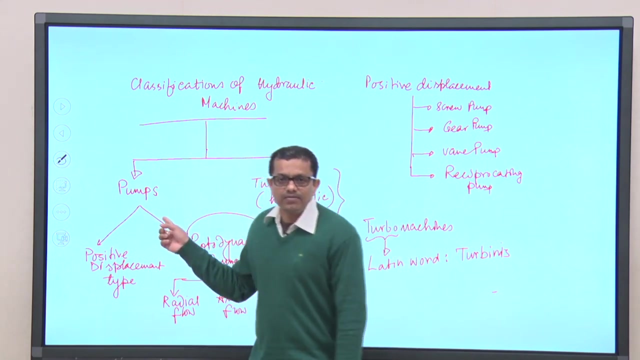 what do we understand? The pumps are the mechanical devices in which mechanical energy, rather the energy coming from the rotating element of the pump, rotating element of the machine, is converted into the stored energy of the fluid right. So that means when we talk about pump, it may be compressor. in case of a compressor, what? 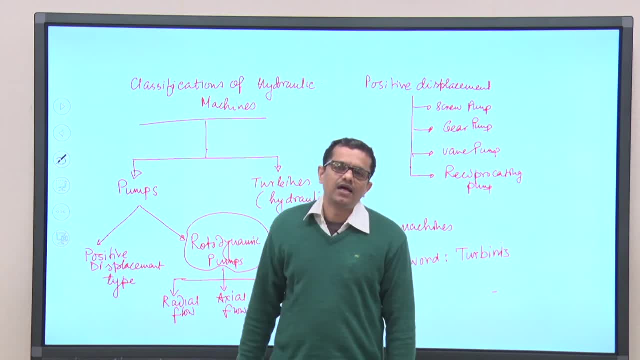 do we? do We increase the pressure of the air, since air can be treated as the air is a compressible fluid. so basically, while the pressure is increasing, temperature will increase. Ok, Ok, that is different tissue altogether. thermodynamics is involved. I am not going to discuss that. 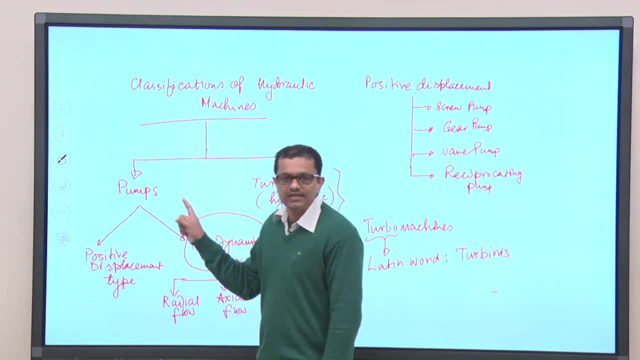 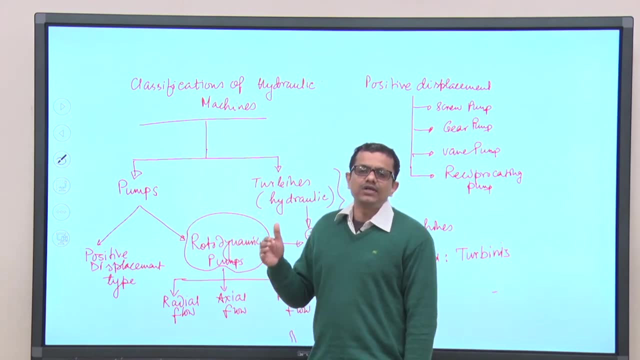 part, but at least here. what should I discuss is that, in case of pumps, mechanical energy from the rotating element of the pumps or machine is converted to the stored energy of the fluid. Stored energy of the fluid. it may be the velocity, that is kinetic energy. 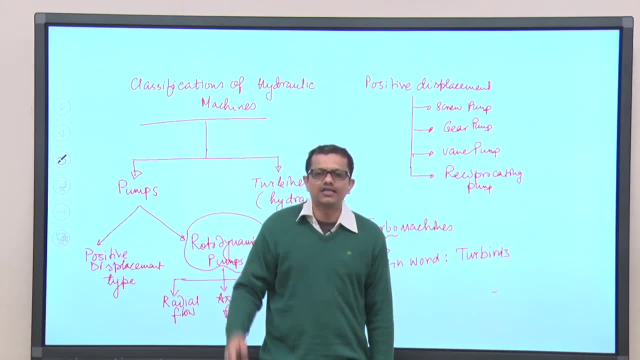 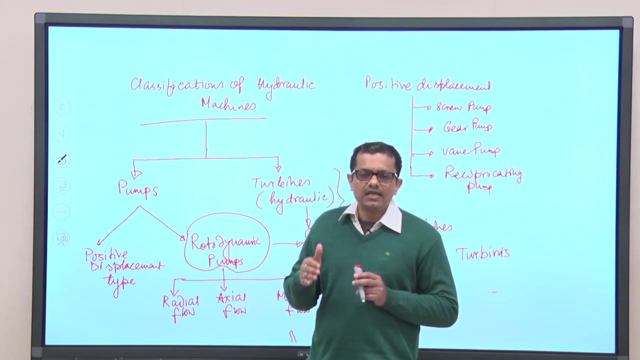 maybe the mechanical energy is used to increase the kinetic energy of the liquid. It is, sometimes it is used to increase thepressure of the liquid. rather, I- I should say the mechanical energy of the rotating elements is used to increase the internal energy of the fluid. 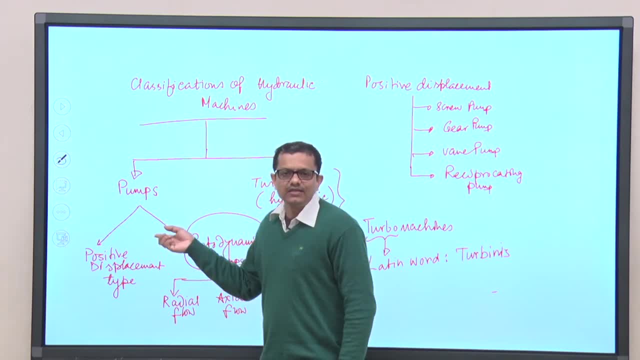 So in case of a pump it is used to increase either velocity or pressure or Tigercount made by connection of positively north wind five p west north, w previous leur dasto mode, combination of these two. in case of a compressor it is used to increase enthalpy. ok. 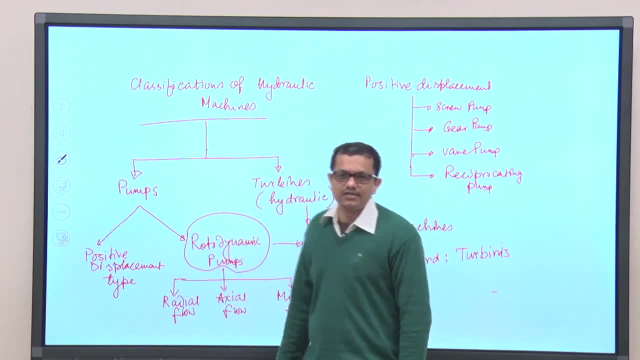 What about for turbines? For turbines, reverse is there. that means we increase the mechanical energy of the rotating element of a rotor right. It is using or utilizing the stored energy of the fluid. We allow fluid to flow from a you know reservoir into the turbine. 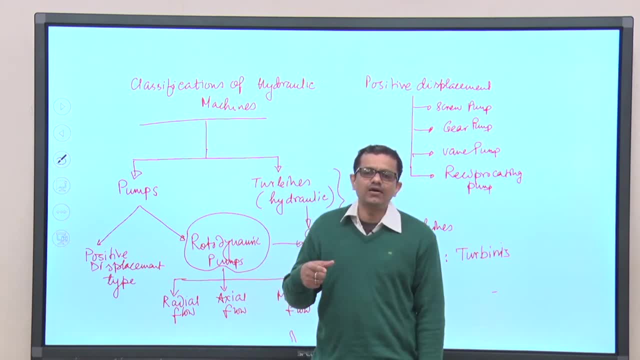 and while the fluid is entering into the turbine, it will allow, by virtue of change in momentum, it will allow, the rotating part of the machines, rotating part of the turbines to rotate and from there we get mechanical energy. ok, So to summarize the first classification, 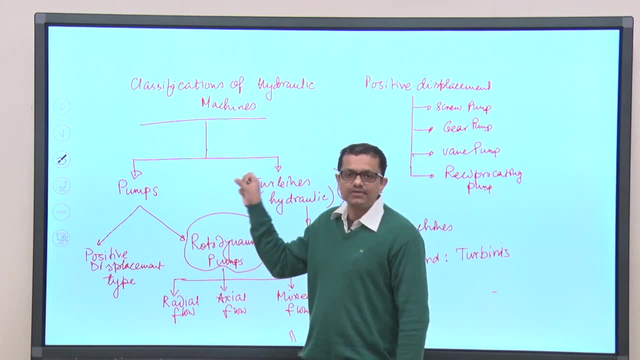 is based on the fact that pumps absorbs energy. So, in case of a pumps, what is done? and for the turbine? So basically, pumps and turbine pumps absorb energy. work is done on the fluid in case of a pumps and in case of turbines, reverse is true. that means fluid does work. 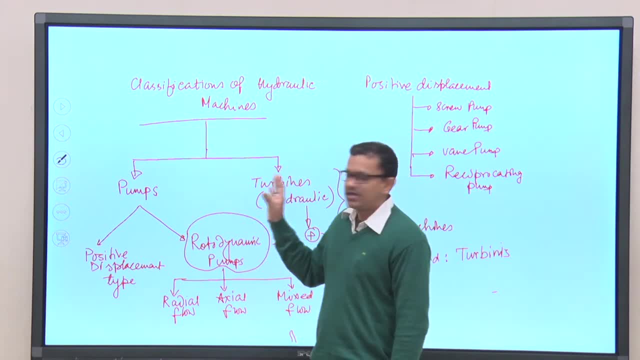 on the machine. ok, So this is the classification. pumps absorb energy. turbines: it produce energy. In case of, I mean I should not say the produce, because energy cannot be, I mean energy is getting converted. rather ok, So in case of a turbines, in case of turbines, the we produce energy. 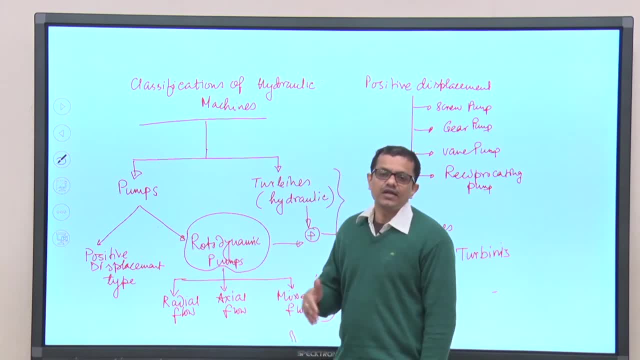 This classification is based on the fact that the working principle of the pumps, So in case of a turbines, in case of turbines, the we produce energy. And finally, the last classification, that is rotodynamic, to the different class of pumps, that is radial flow, axial flow. 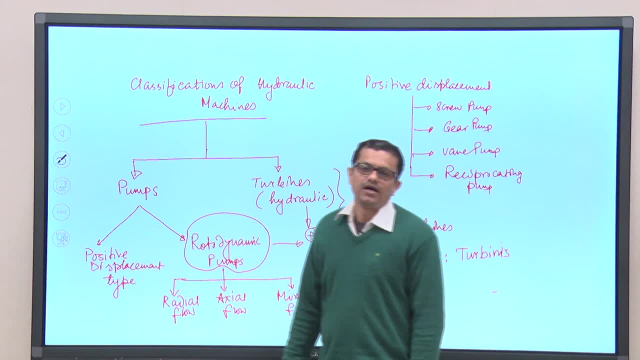 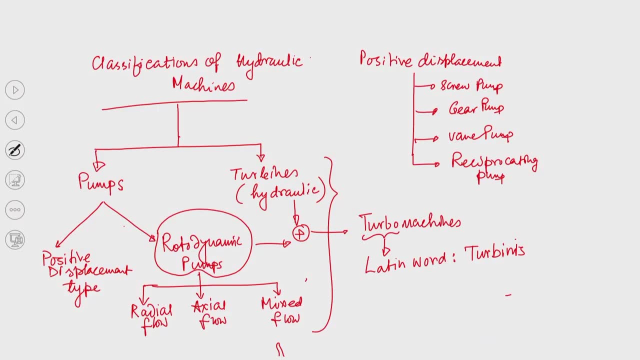 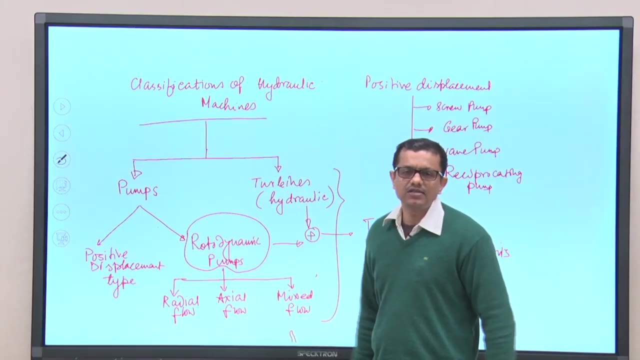 and mixed flow. this depends on the direction of fluid flow inside the pump. ok, So, and we also discuss that- turbines and rotodynamic pumps- these you know machines are sometimes known as not sometimes they are also known as turbo machines. The word turbo is coming. 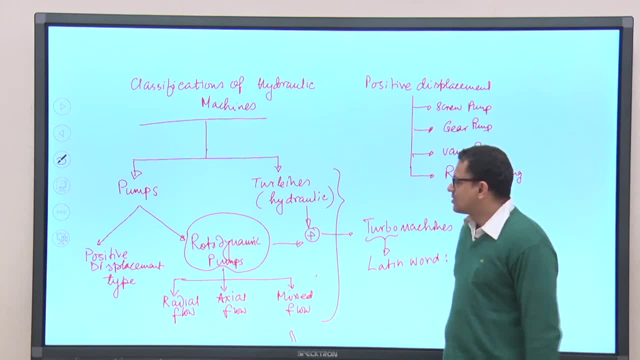 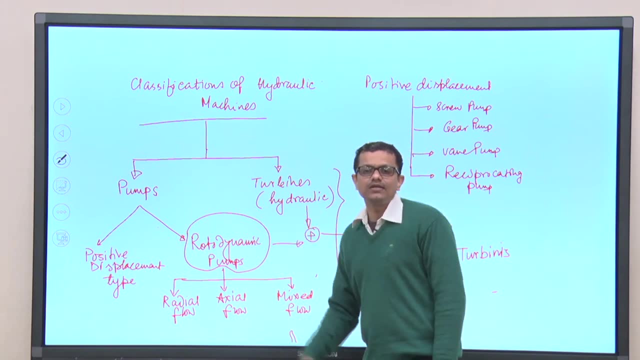 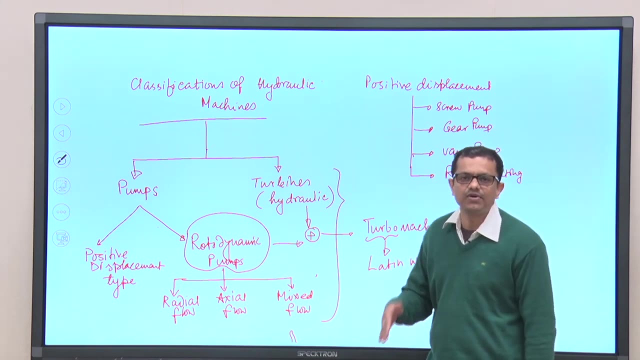 from Latin ladder a over turbine is that is swirling action. So in all these machines, whether it is rotor, dynamic pumps or it is turbine, the rotational effect that is, the rotor will have rotation and by virtue of which we can have energy conversion, whether it is from fluid to the 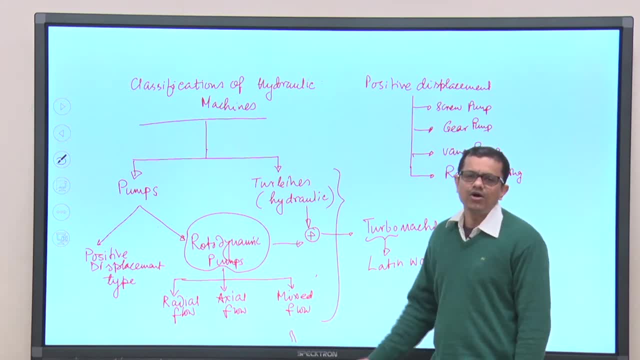 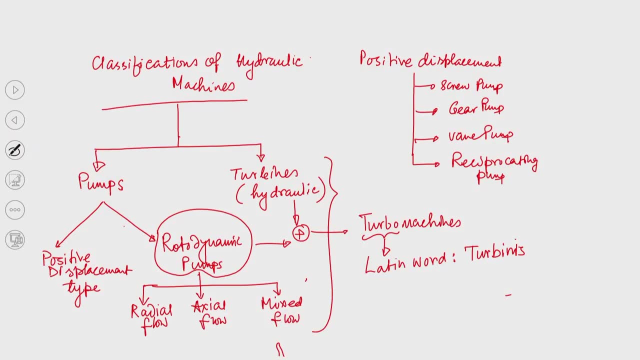 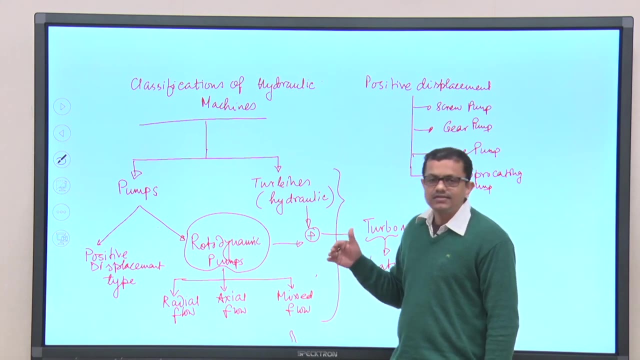 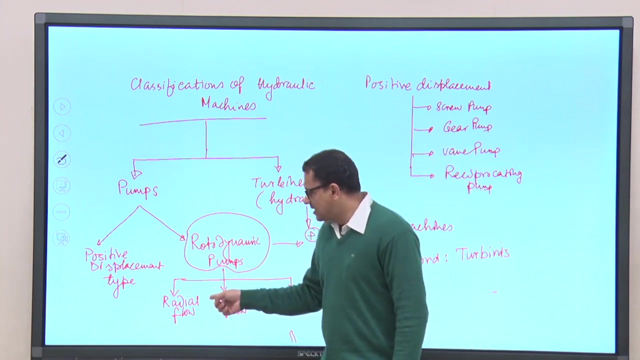 mechanical, mechanical component or from mechanical component to the fluid. Now we should go to see that the classification that we did based on the direction of fluid flow, and since I will be focusing more on the hydraulic machine, So slowly, I will now move to see that this classification- radial flow pump, axial flow pump, mixed flow pump. 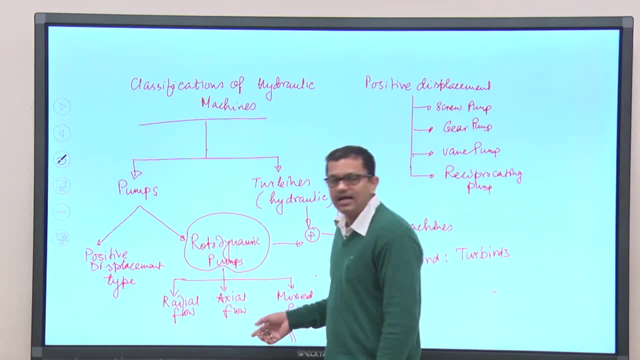 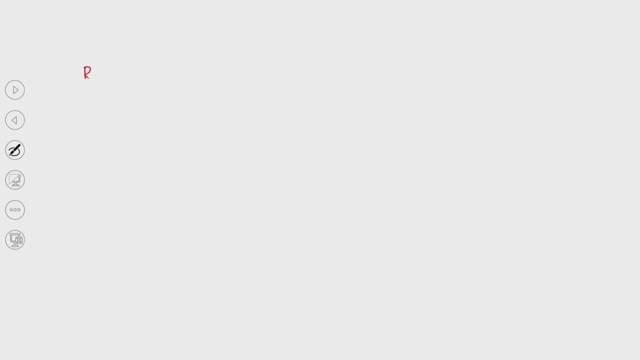 So we also need to discuss that these machines are definitely have a few important applications in different areas And we should at least identify, we should know in which area which type of machine fits well. So if we now try to discuss that first, this radial flow pump: radial flow pump. 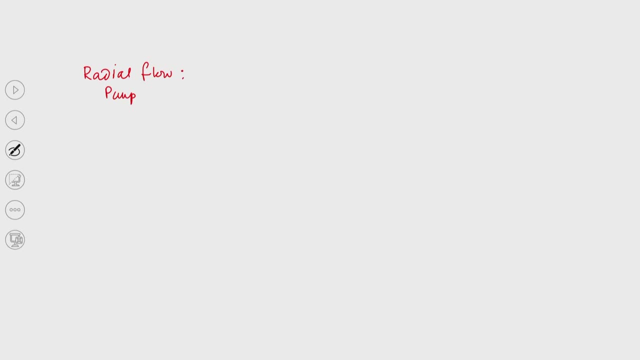 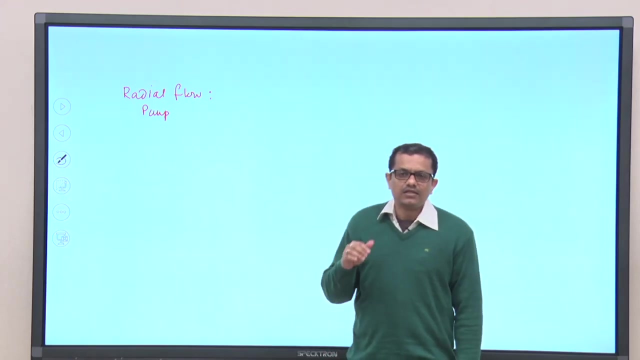 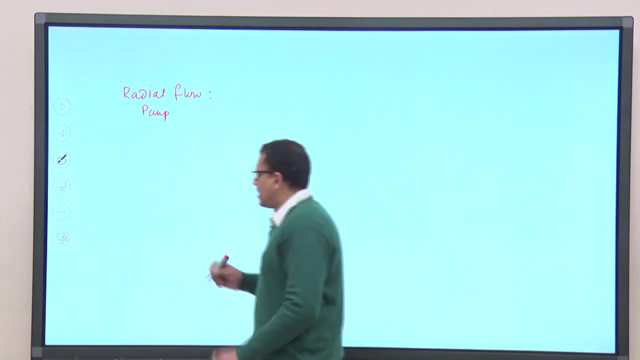 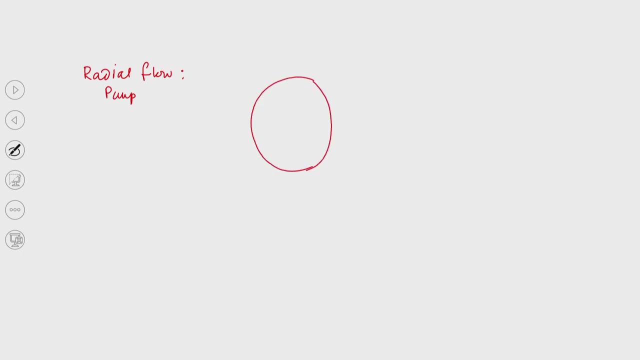 as I said, you that. So this classification is based on the direction of fluid flow inside the machine or pump. Radial flow pump: the flow of the pump, flow of fluid inside the pump, is perpendicular to the direction of axis of the pump. That means, if I try to draw a schematic, So I 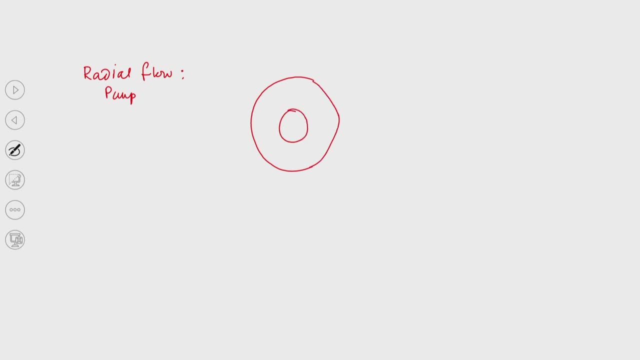 have a small callage And if we try to draw, you know if we Thank you. So this is the axis of the machine and this is the rotating part and this will have rotating rotation, right. So, in this case, what we can see from this diagram, this rotating part, which 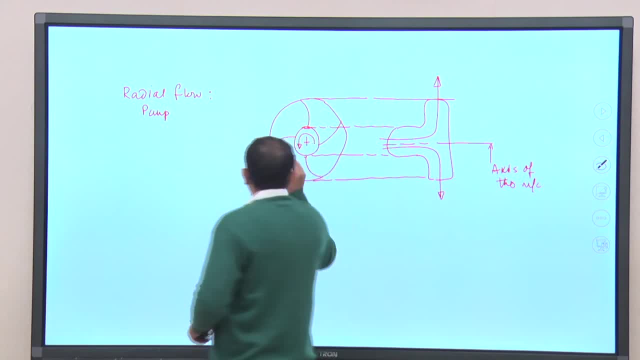 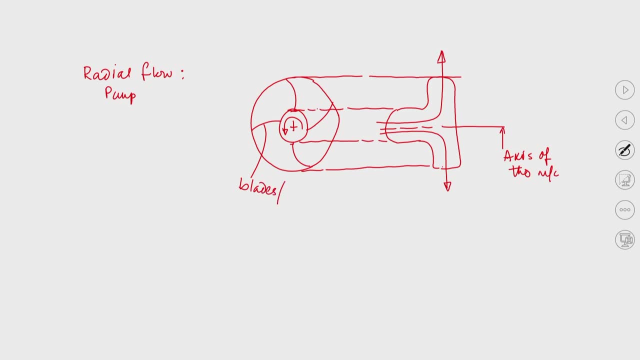 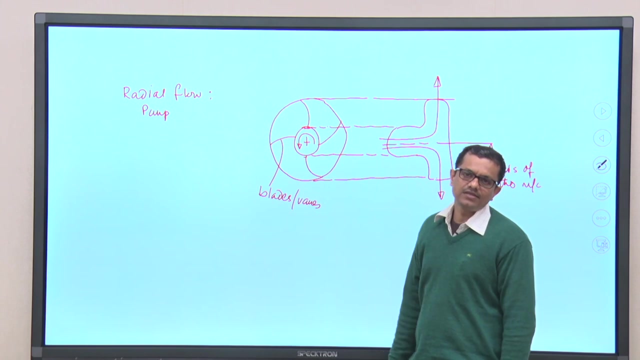 is known as impeller. I will write that these are known as blades or vanes. So these are known as blades or vanes, and this you know. I have drawn two concentric circles. the inner one, Which is having smaller diameter, is known as hub. So this hub. So this is known as. 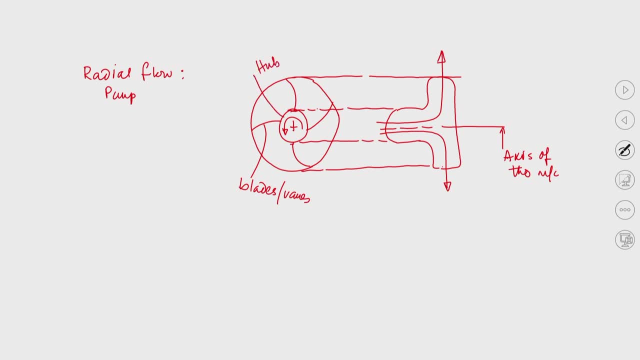 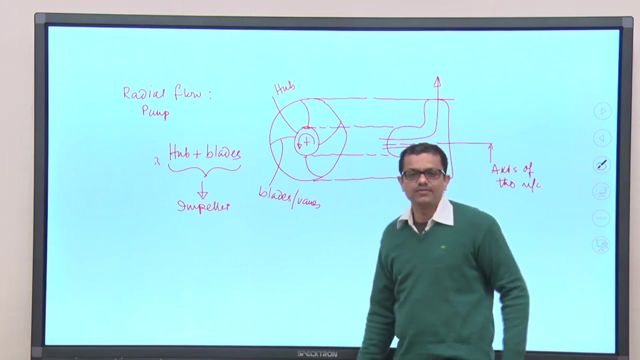 hub right Now, hub plus blades. I will write here this hub plus blades, this hub plus blades. it is known as impeller for the perm, So impeller. we will be using the word impeller very frequently in the in this context. So what I am telling hub plus blades will have. 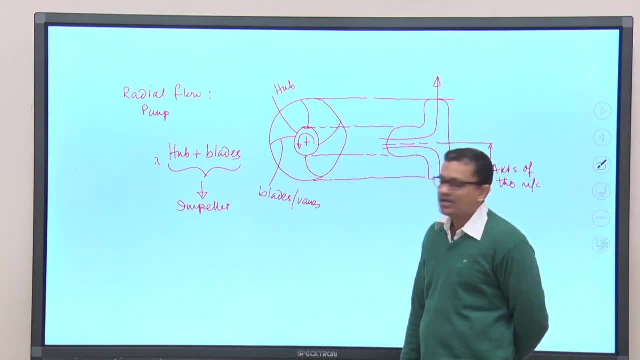 a few blades, depending on the requirement that we will discuss slowly that the number of blades Will be selected based on the requirement of the energy that we need to convert. So this hub plus blades, which is known as the impeller, so this impeller will have rotation. 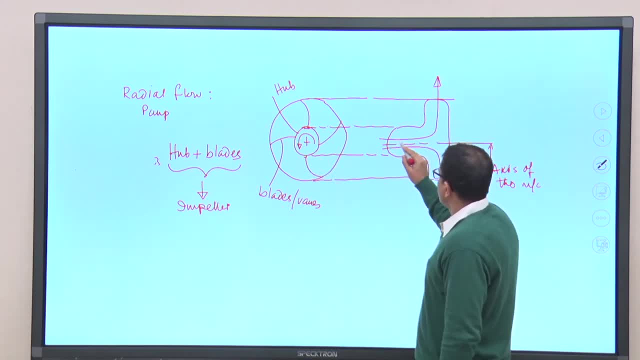 and the. this is in. let now what we can see. I wanted to discuss about radial flow perm, So you can see the direction of flow inside the impeller, inside the perm which is perpendicular to the- you know- axis of the pump. Following here we will have the. now there is the sinister. 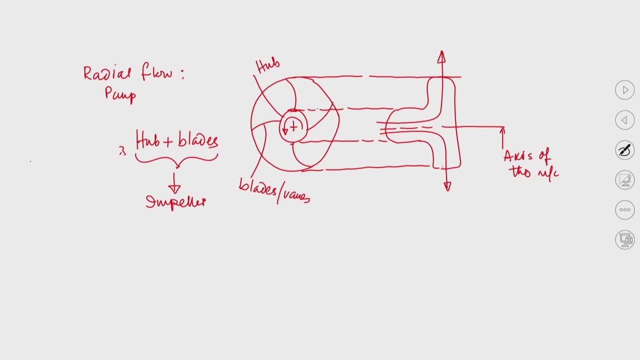 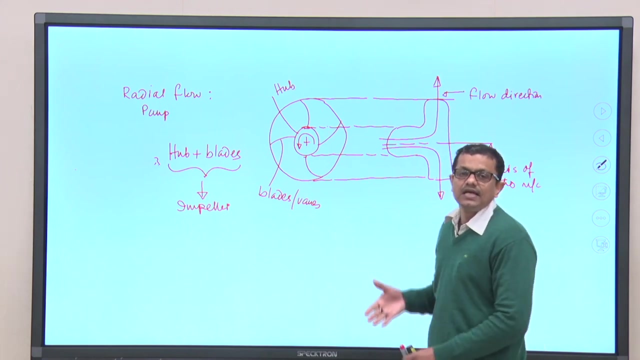 you know, axis of the machine. So this is axis, axis of the machine and this is the flow direction. So this is flow direction and this is why it is known as radial flow pump. that is, radially outlet. So we can see, this is the flow, is in the radial direction. Sometimes, 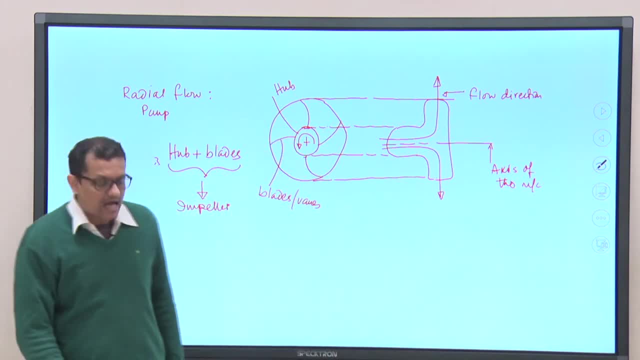 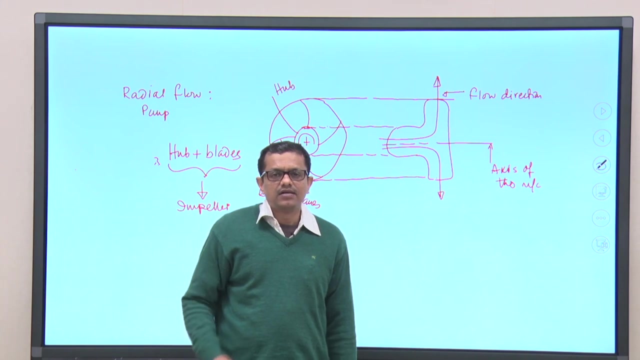 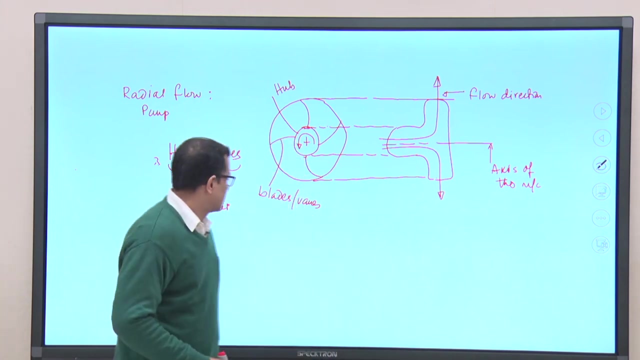 this type of pumps. I mean this type of pump is known as centrifugal pump. If you, you know, consult any text books, you will find that the say the words, you know the words: the centrifugal pumps. the centrifugal pump is used frequently, So sometimes this radial pump is used frequently. 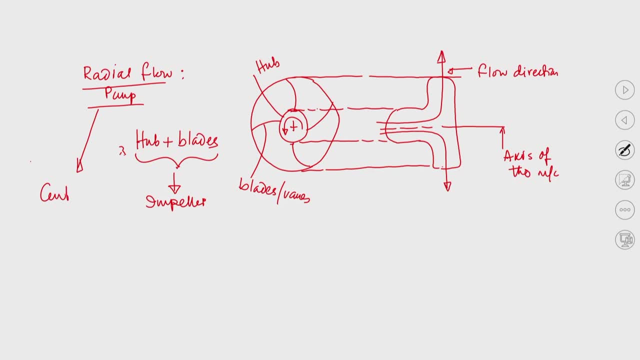 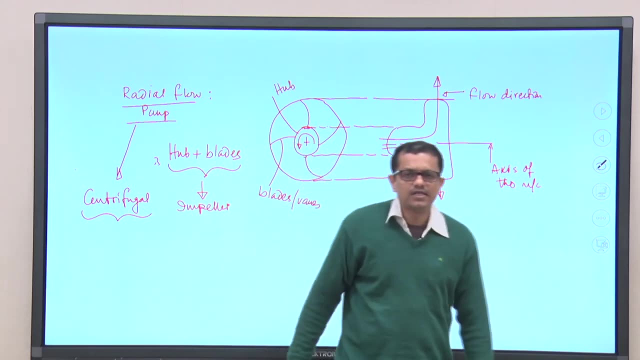 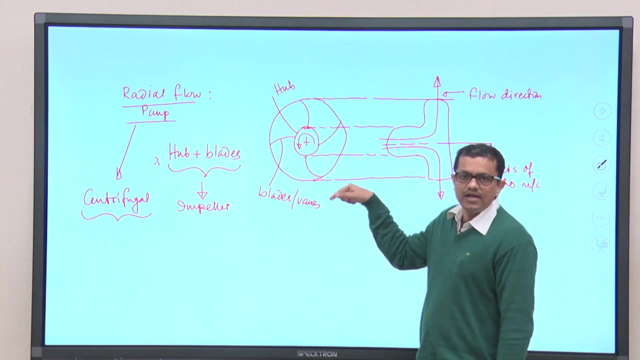 Radial flow pumps are also known as centrifugal pumps. centrifugal pumps- I have little bit, you know reservation to say exactly the pump name of the pump, as the centrifugal pumps by because the you know energy, that is when the wheel, the impeller, is rotating half plus. 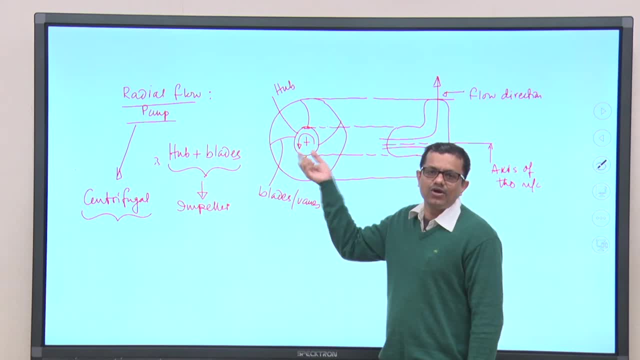 blades. So this will be driven by either electric motor or diesel engine. Now when the impeller is rotating, that means the mechanical energy is imported to increase this. you know internal energy of the fluid. So by rotating the impeller we are trying to convert mechanical energy to the internal. 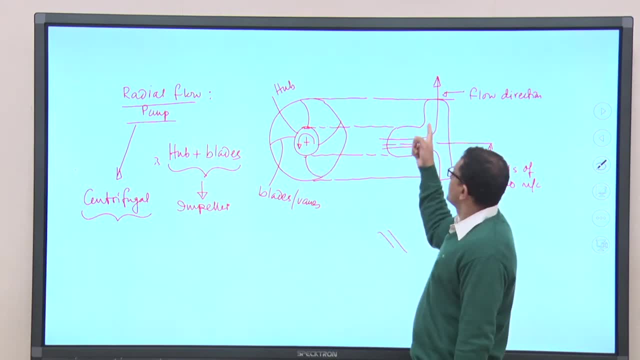 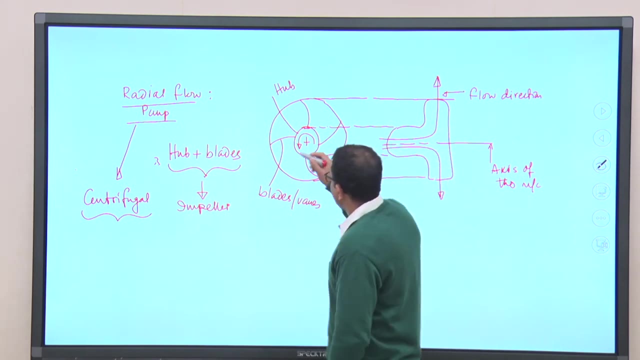 energy of the fluid and because of this we are getting, you know, high pressure of the impeller or high velocity of the liquid which is coming out from the pump right Now when this is coming out. so this is rotating and the liquid is try to coming, come out in. 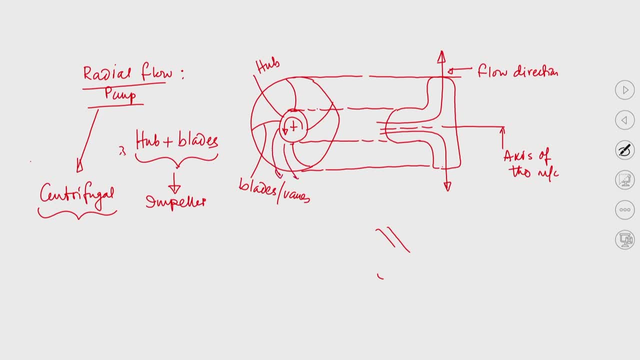 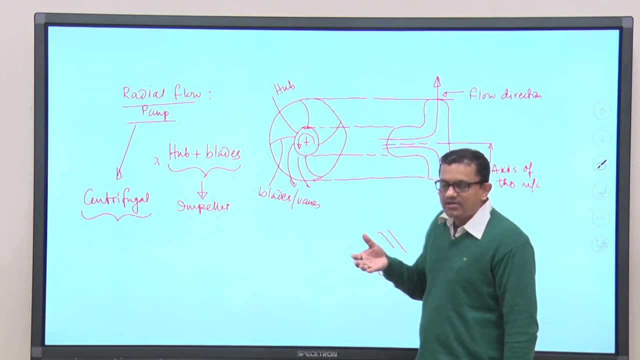 from the passage between two consecutive blades. So the centrifugal action is there and the liquid- I mean the water which is coming out from the pump- is having high velocity and pressure, and as if the centrifugal action is responsible to increase this, you know, pressure or velocity. that is why it is known as centrifugal. 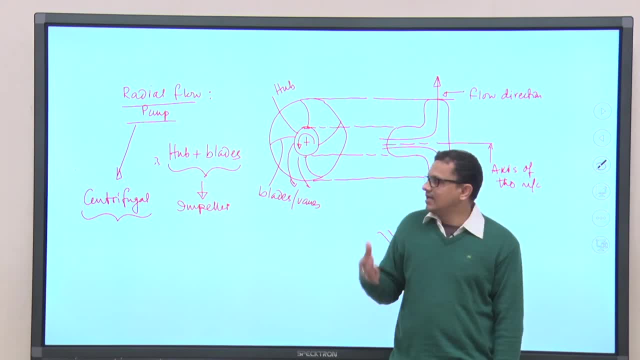 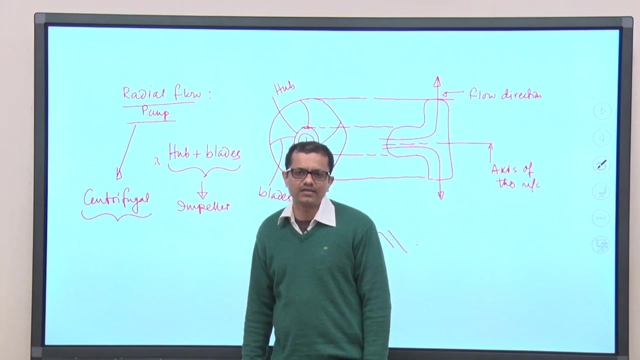 pump. But we will see that the there is one another type, there is another type of pump in which centrifugal force is still acting and if we need to say a particular pump To be the centrifugal pump because of the, because of the presence of centrifugal action, 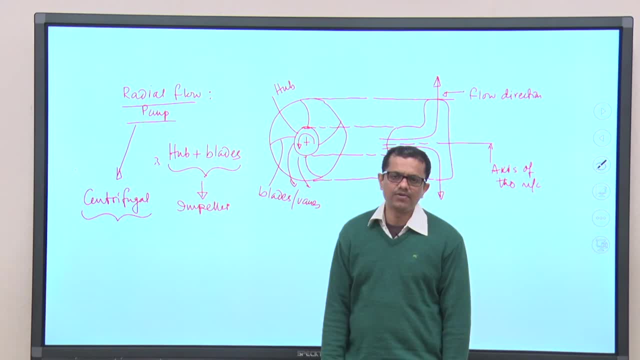 then also we need to call the another you know type of pump to be the centrifugal pump. So I should say, instead of calling this pump as the centrifugal pump, it is advisable to call it radial flow pump. but centrifugal pump is, it is the commercial name. 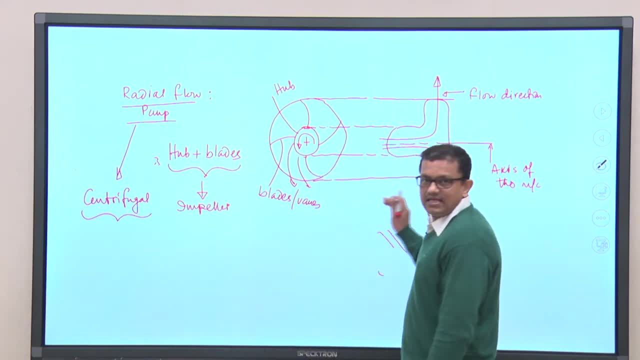 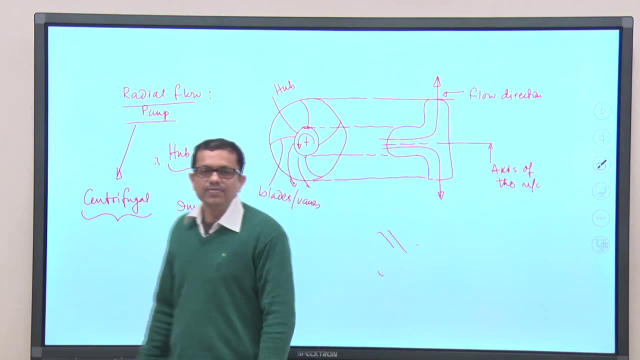 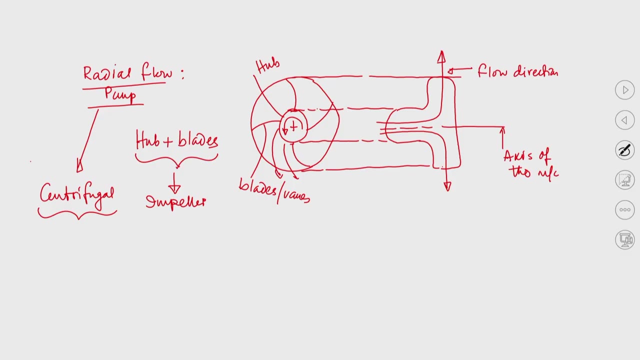 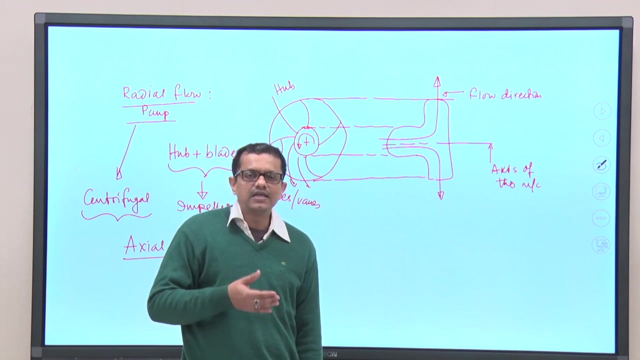 Okay, So this is the case, that in this case the direction of flow of fluid inside the pump is perpendicular to the axis of the machine. So next I will talk about axial flow pump. A radial flow is in the axial direction, so that means flow of fluid inside the pump. 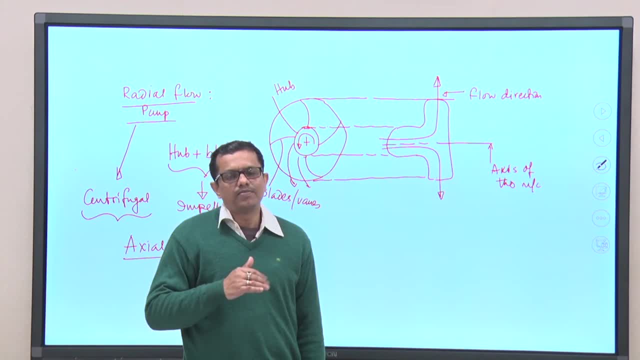 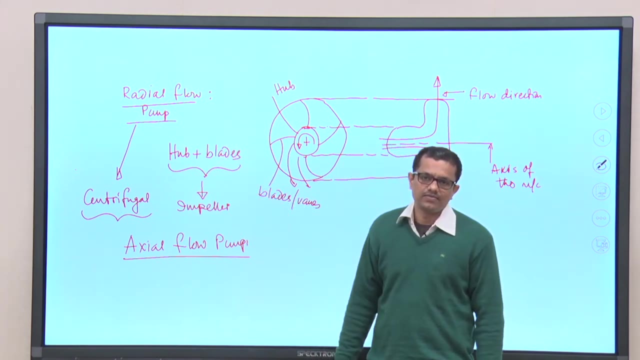 is parallel to the pump axis, and these types of pumps are known as axial flow pump. By the way, I should say that the radial flow pumps are suitable in places where we need to aisle milk heaps своего instrumental. 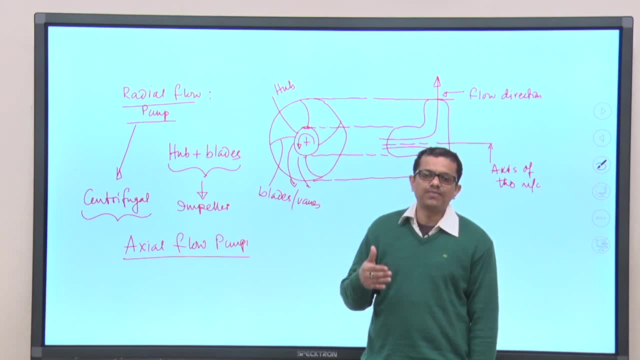 Then I am telling. the purpose of installing the purpose of the pump is to provide head and discharge. So that means we need to supply water from one place to the other place, that is discharge, that is known as discharge. and if we need to supply water from a first floor to the 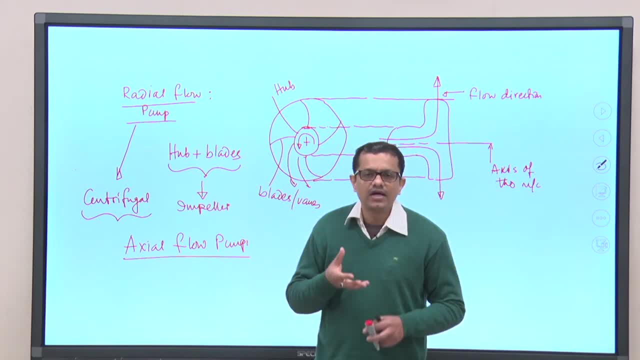 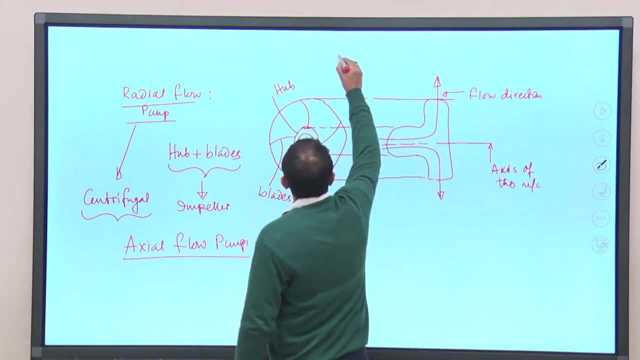 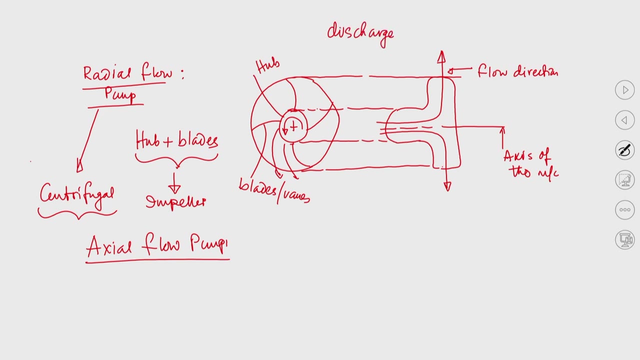 top floor in a multistore building. definitely, we need to develop head by a pump. So these two important parameters- one is known as discharge, that is cube, denoted by cube, and head, that is h- these two parameters are very important, depending on the requirement. 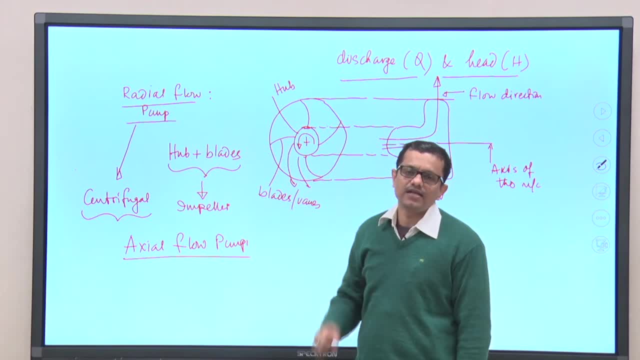 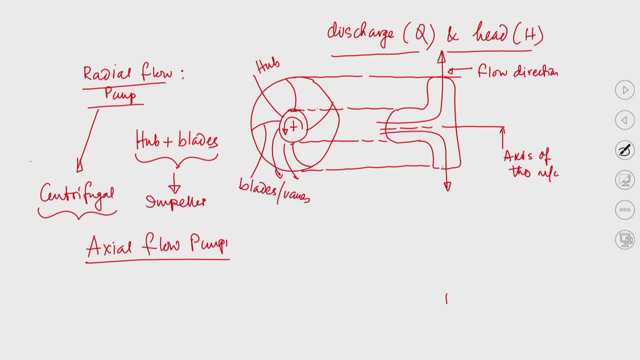 of these two parameters, these two quantities, we need to select which time, which type of pump will be. you know best for a particular application. Radial flow pumps are suitable in those applications where we need to supply low to moderate head. So basically, I am writing this, pumps are? you know I am writing over here. 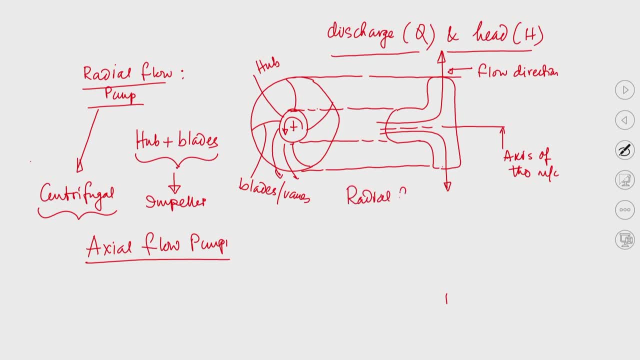 Radial flow pumps suitable for low to moderate cube. So this is the first point, So this is the second point, So this is the third point, So this is the fourth point, So this is the fifth point. 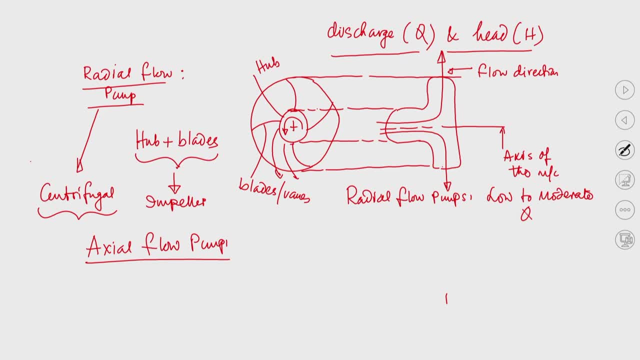 So this is the fifth point. So this is the eighth point. So this is the sixth point. So this is the sixth point. So this is the distance from the used water: 250 meter, Jesus fuck. Based on the flavor, the concentration of water for a specific time in the location. 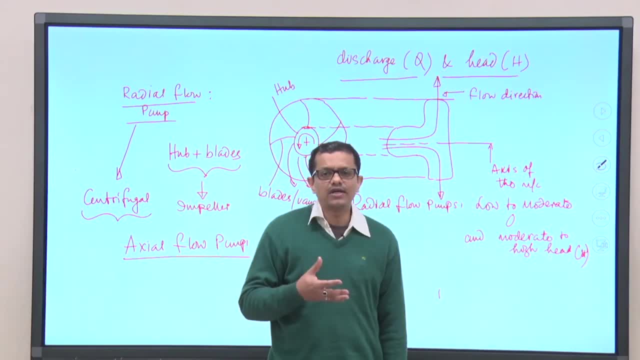 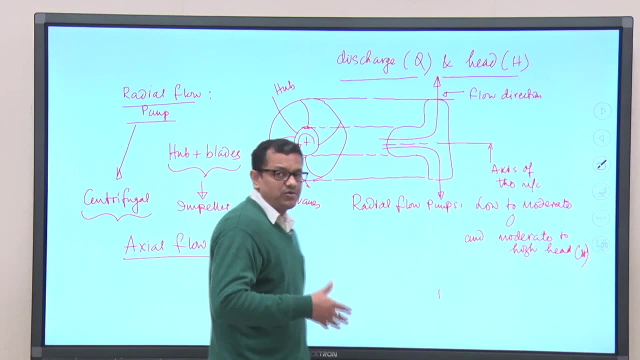 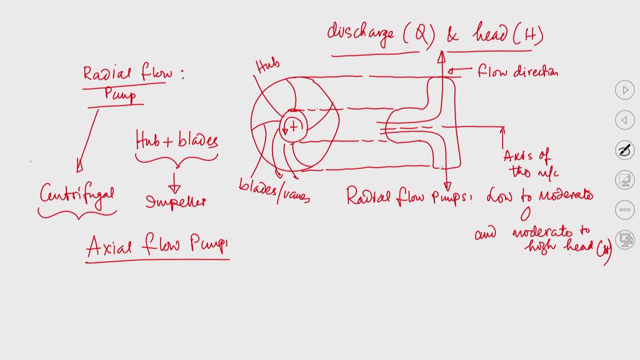 of discharge process in applications where you need low to moderate discharge against moderate to high head. right Now, if we, you know, move to discuss about the axial flow pump. So, axial flow pump, basically I am writing the, I am drawing the schematic here. So in this pump, what we can see. So this is the incoming flow, this is the incoming 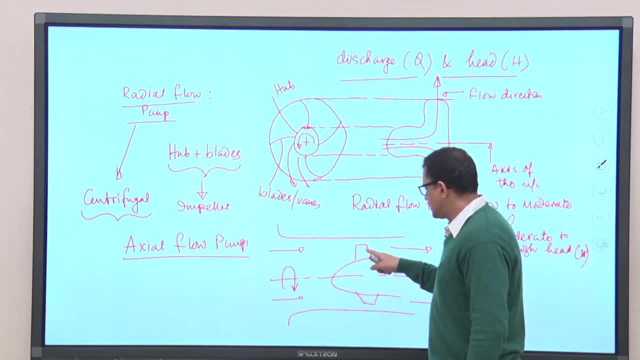 flow. this is the impeller, So these are the blades and this is the. you know how much the hub and hub plus blades impeller. So impeller will have rotation. incoming flow will now have movement while they are approaching the pump and leaving the pump, which is parallel. 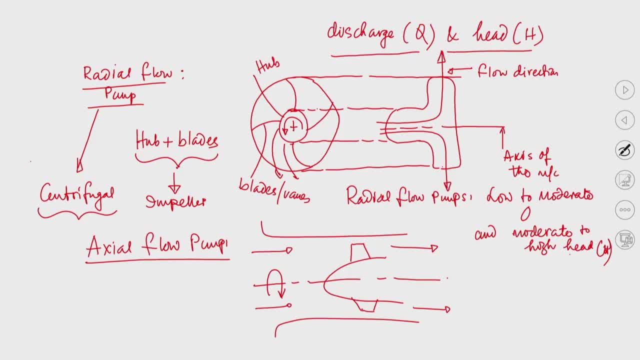 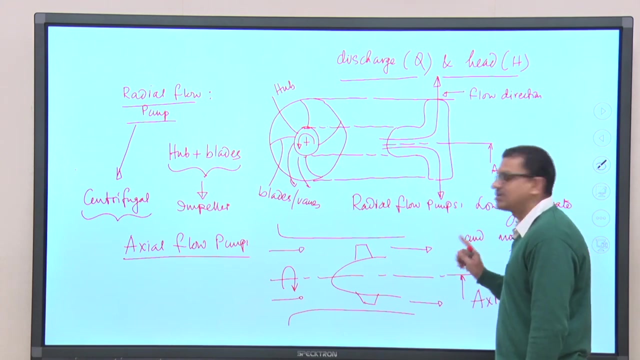 to the axis of the machine. So, basically, this is axis, this is axis of the machine. Okay, Okay, So the what we can see? that the flow direction, the flow of fluid in the machine is in parallel to the axis of the machine, and that is why these machines are known as axial flow machines. 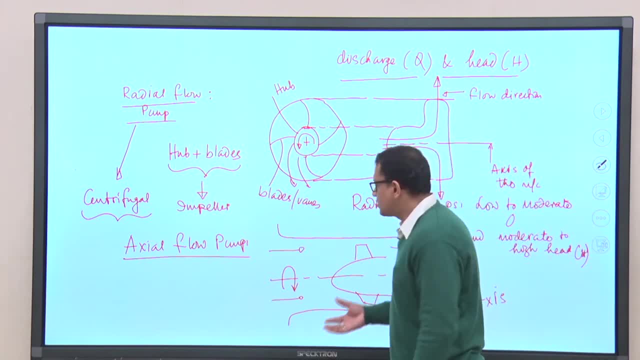 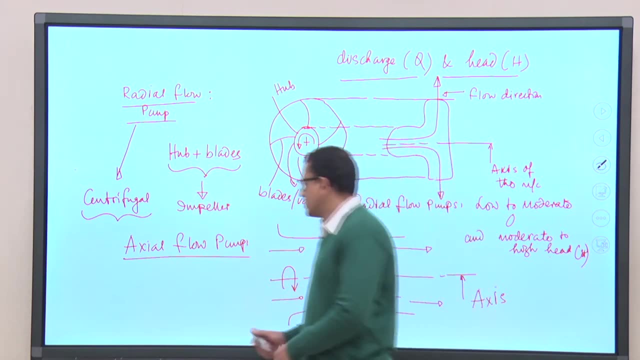 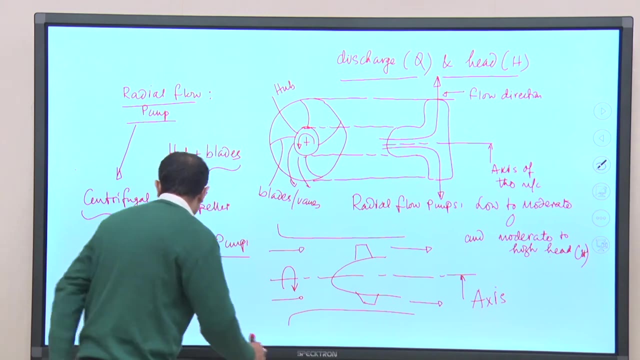 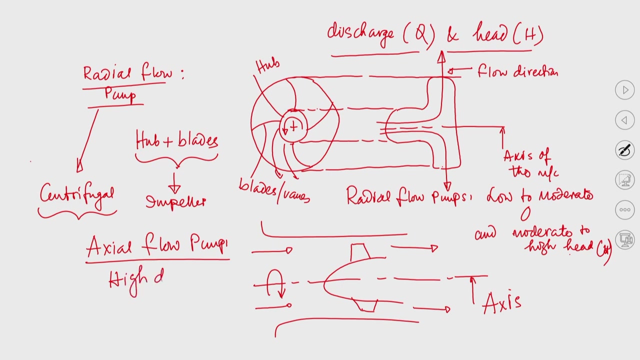 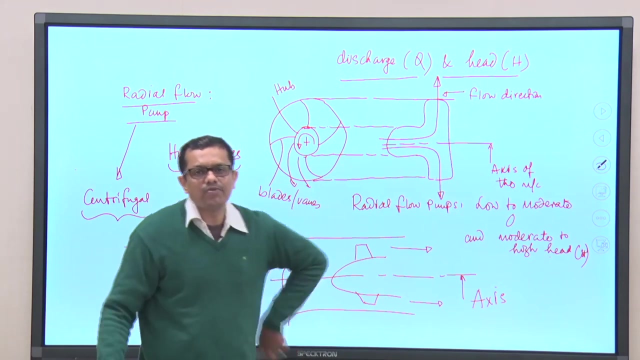 ok, Again, we need to know at least these machines where fine you know applications. So these machines fine applications in places where we need to supply, you know, high discharge, which is very important. For example, an low head that means when you need to supply huge quantity of water against. 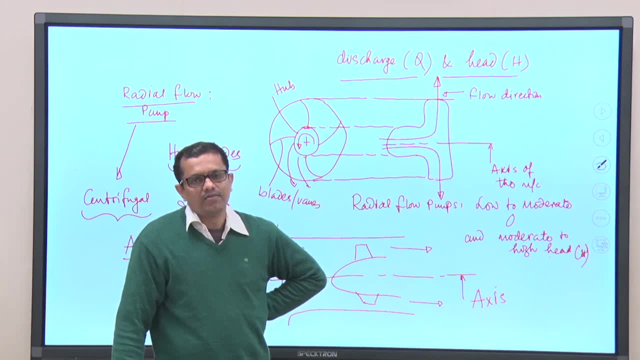 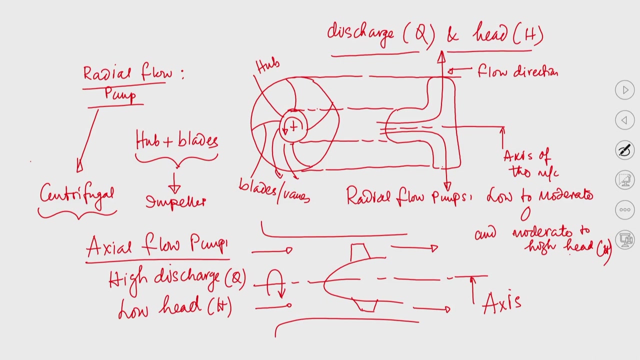 a low head, axial flow pumps are much more suitable. That means what are the typical applications? agriculture, coal mines, where axial flow pumps are much more suitable. We need huge quantity of water at a reasonably low head, So that means axial flow pumps are used in. you know I can write applications- coal mines, So that means axial flow pumps. 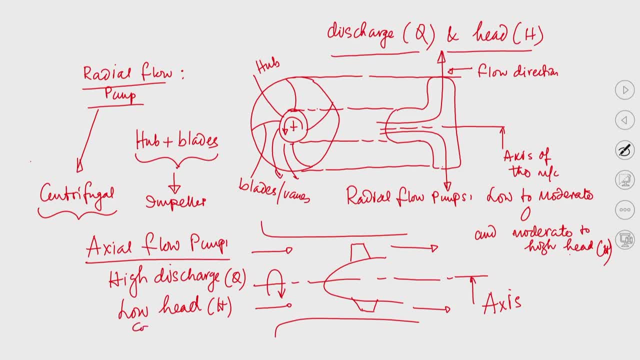 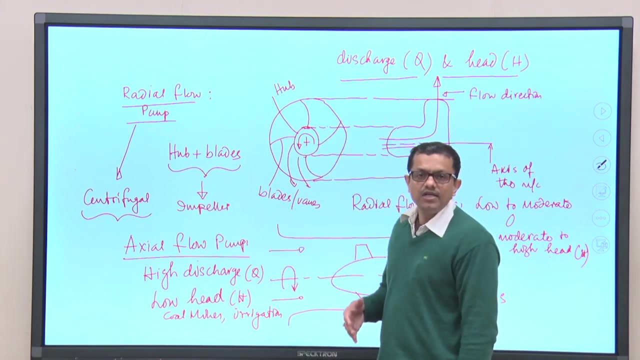 are used in. you know I can write applications: coal mines, So that means axial flow pumps are used in. you know I can write application: coal mines, So that means axial flow pumps are used in. you know hay 심 cultura, or universal mills. 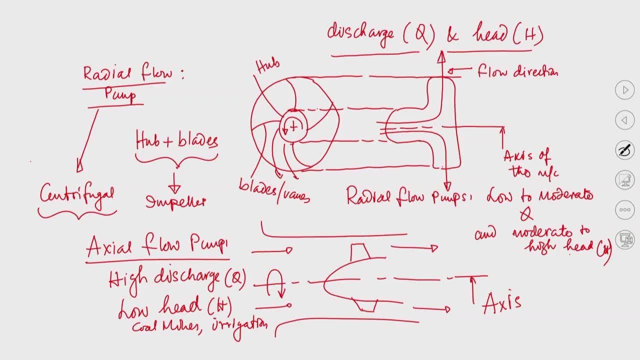 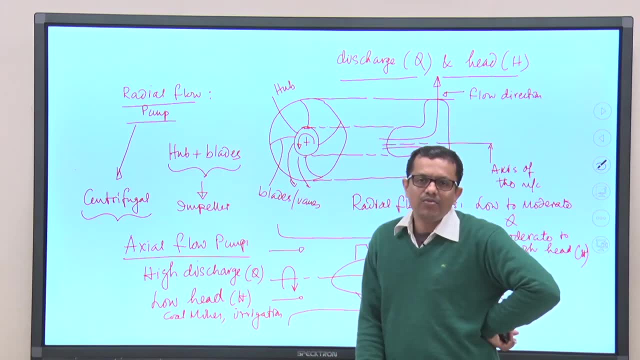 Then again we need asked at least 3 to 4 man Caucasian oil. so again you canCEUISMA family, but increasingly it may also may increase with use. Where again you canCEUISMA family, maybe also Korea. So that means axial flow pumps are we need? 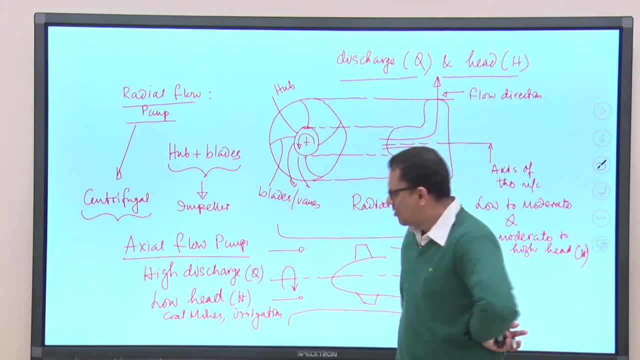 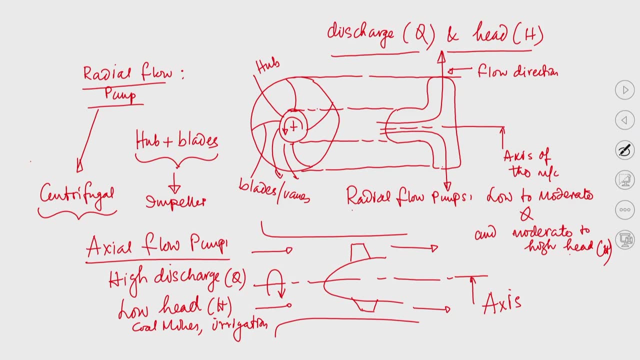 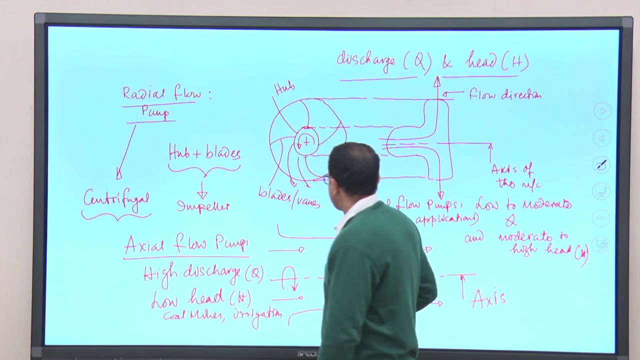 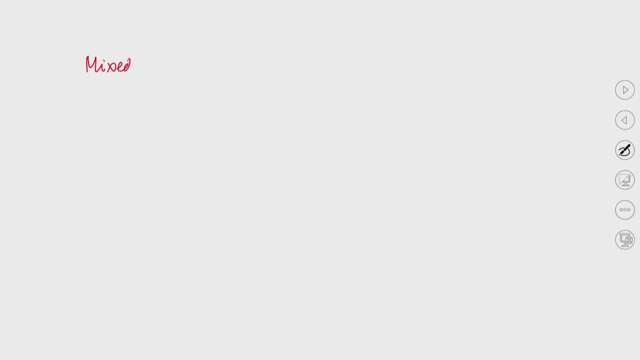 and sometimes they are also used in different process industries. So I am writing radial flow pumps used in domestic applications mostly, and then we are left with the last one, that is, the mixed flow pump. So finally we will have mixed flow pump, So we can say that. 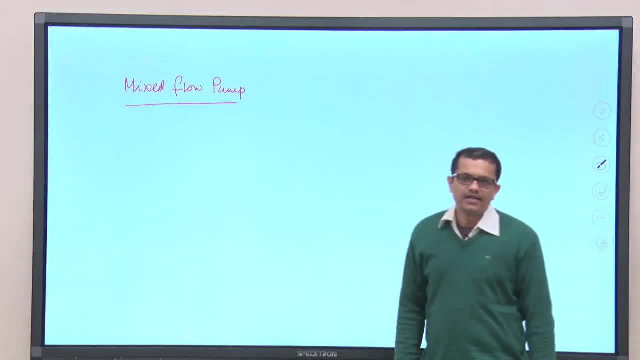 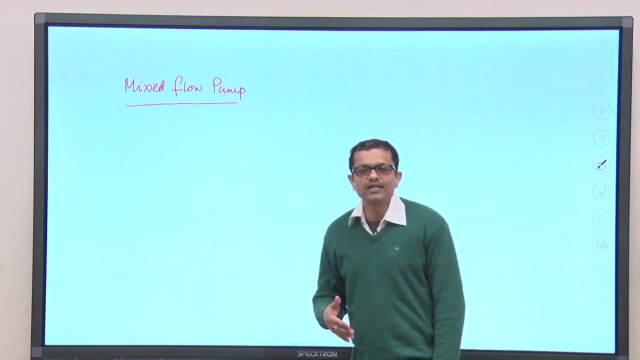 in a mixed flow pump. basically this is the combination of the first two, that is, flow is neither purely radial, it is not purely axial. So in a radial flow pump we have seen the flow of fluid in the pump is in the radial direction, that is, the direction is perpendicular. 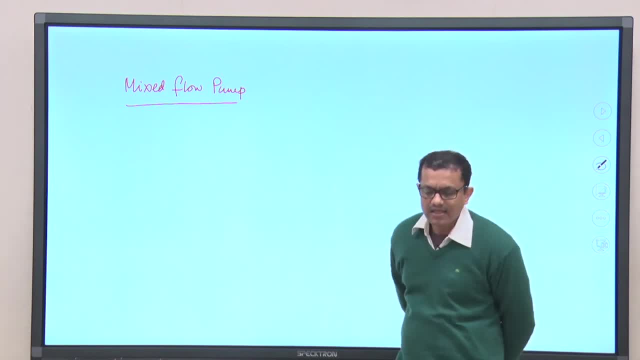 to the axis of the machine. In case of axial flow machine, the flow of fluid in the pump is parallel to the axis of the machine. For the mixed flow it is neither purely radial nor purely axial, that is, combination of these two. So that means if we try to draw the 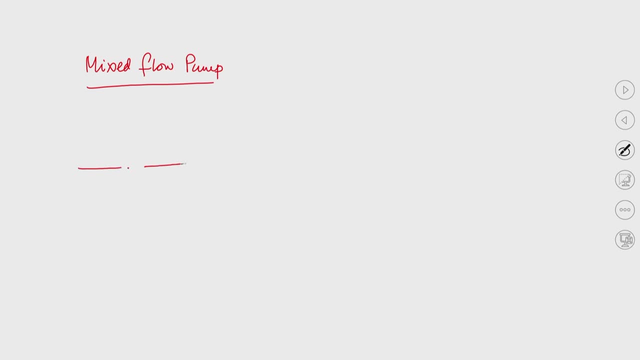 schematic ktorh only by 노�s. Of course, you see it on the screen. So this is z direction, this is theta direction and this is r direction, and we can see r direction. thus, this is z direction. that liquid is coming like this. Now, what we can see from this figure is that this: 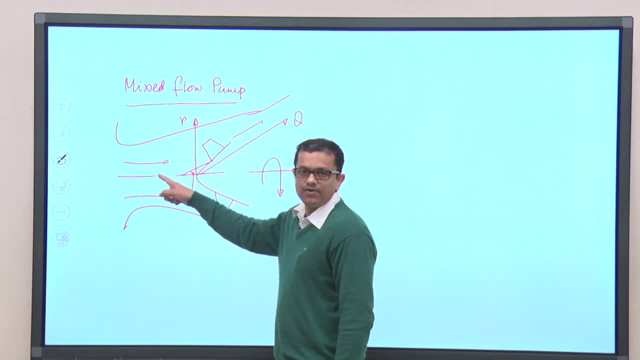 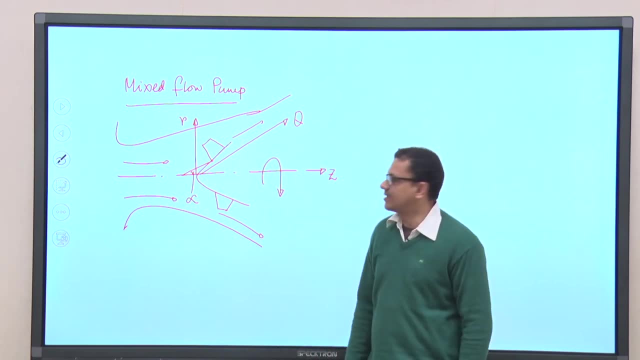 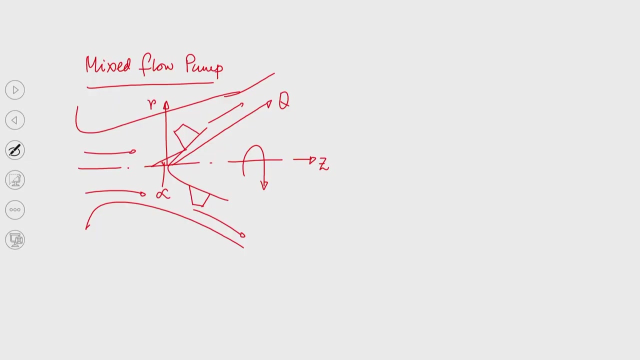 is pump impeller blade plus half incoming flow which is approaching to the pump is almost having axial direction. I mean direction is parallel to the axis of the machine. So this is axis of the machine Now, when we are getting flow, rather when it is approaching. and finally, 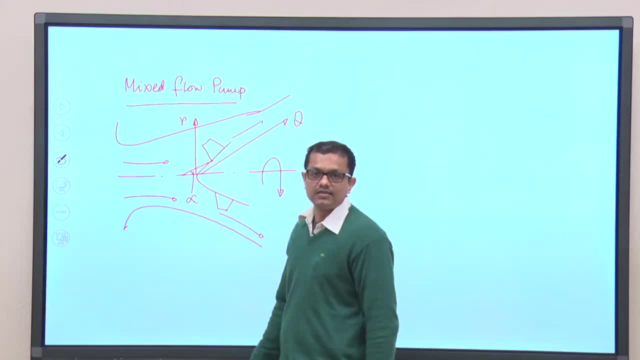 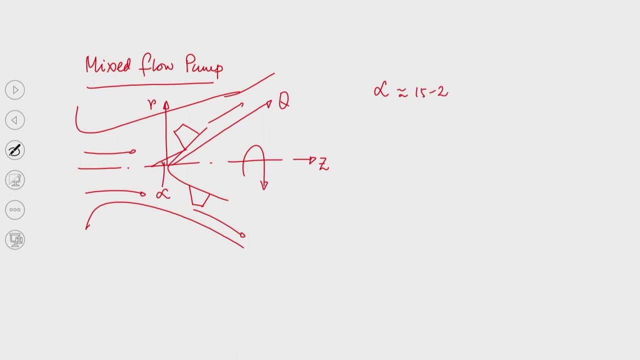 it is leaving the pump. we can see the direction of the flow is getting change. It is not purely radial nor purely axial, and it makes an angle, alpha, which I have shown over here Now. this alpha, it is 15 to 20 degree the angle. If alpha is 0, then it will be purely 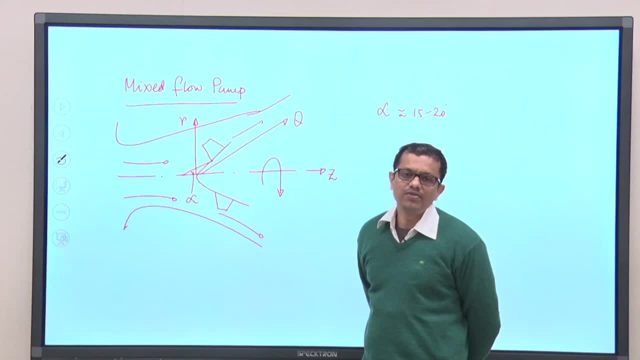 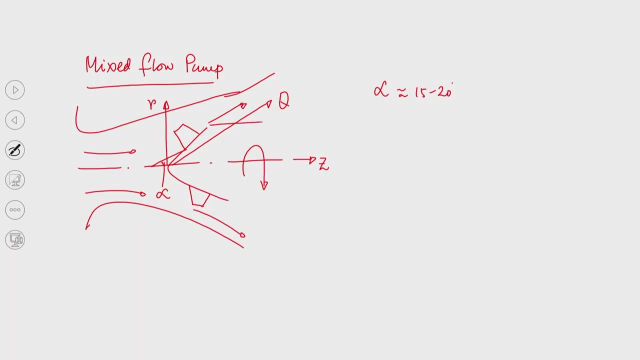 axial flow machine. If alpha is 90 degree it will be radial flow machine, Since alpha is in between. so we will have two different components. I mean, if we try to explain so velocity you know we will have. So we have two different components. One is you know v? r, another is v? z right. So 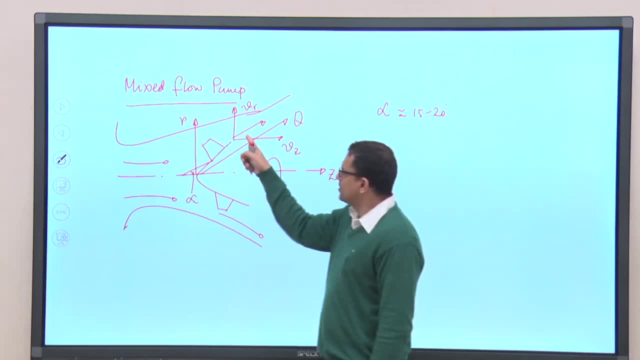 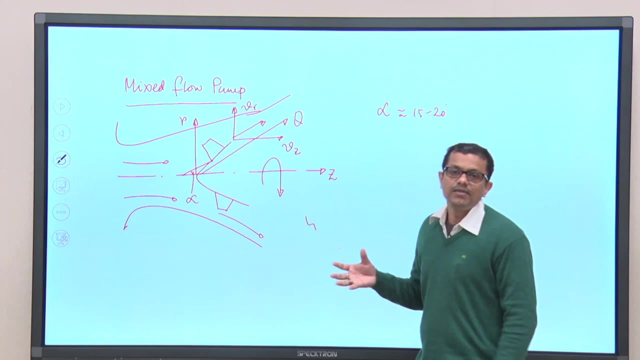 we have two components. The flow which is leaving the pump is having two different components. One is in the radial direction, another one is in the axial direction. So this is not purely radial, not purely axial, and this type of pumps are known as mixed flow pump. So 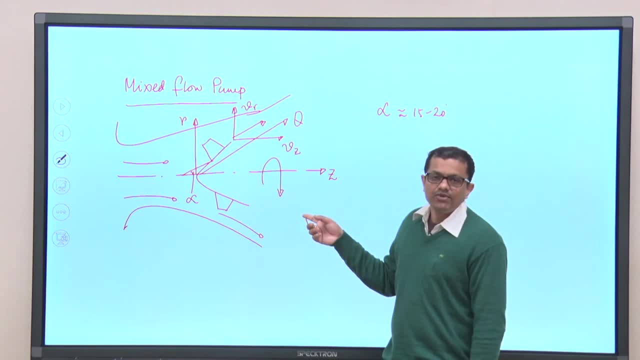 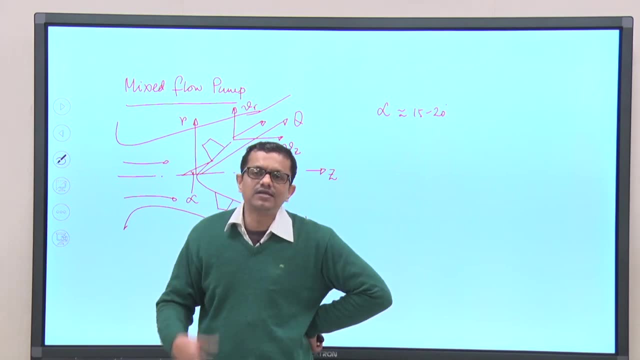 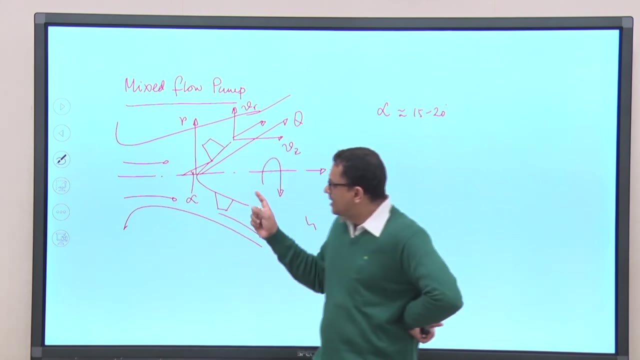 the point that I was talking about in this case also, you can see the radial component is there. So if the radial component is there, that means there will be a centrifugal force. It is not purely axial. So centrifugal force is still there in this pump and which is responsible. 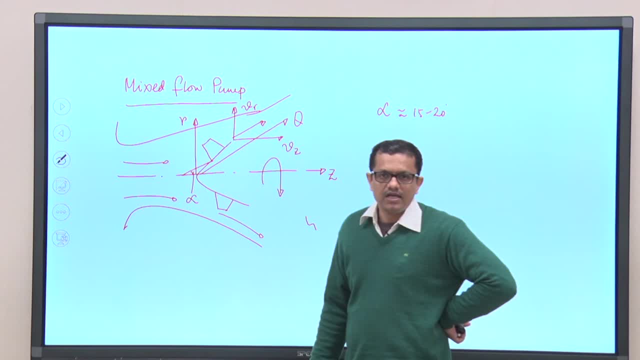 for the rise in pressure using this pump. If the presence of centrifugal force is rising, then it will be a centrifugal force. If the presence of centrifugal force is rising, then it will be a oxidised carbon, So it will rise to hit the legs. the função of centrifugal. 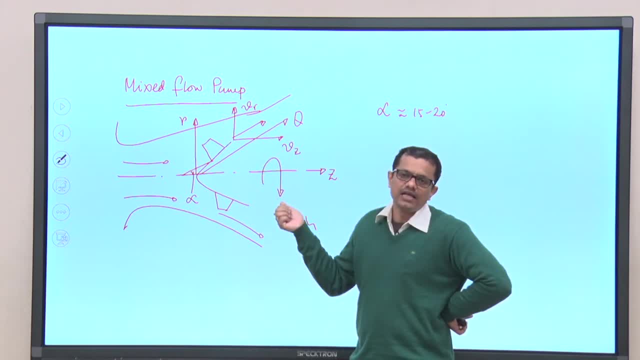 force and it will stretch the legs. the position will be a rotating holder in this. recognize the flow and addition of vibrations, fertilization. So the current compared to current, before all the otheronal movements Which you can see here. we did not remember this is the gebengetge cabinets That there. will be a flow, thisads purposely. this has two critical parts. One is Ok, So basically, down here is thewon to x term itself, So we have aepsic dav. ㅋㅋㅋ. down here is the liquid flow plate here. So, to see this, this will say how the current flow will be in the 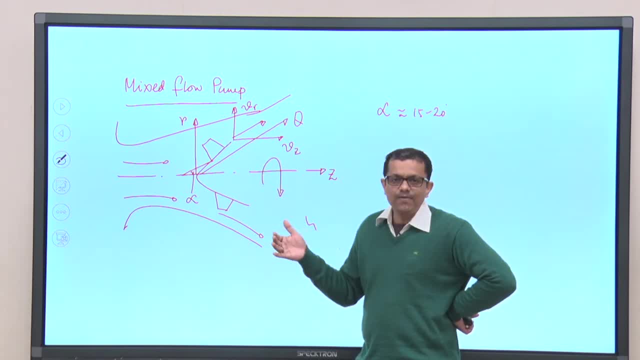 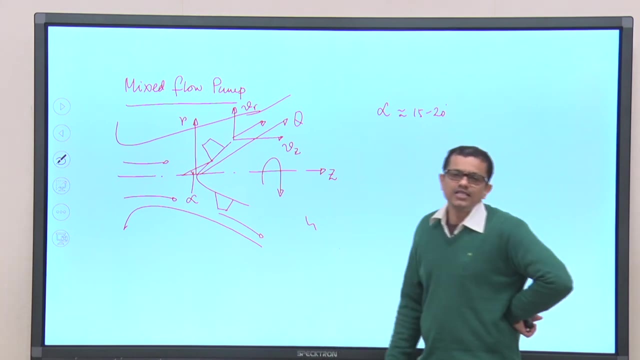 industrial does it And there will also be a pressure, tau x, del x which occurs from the tanks back to the back in the industrial. moto 마 options like example. So these are basically in flow direction is nor completely axial nor radial and these pumps are used in the condensate cooling in a in a steam power plant, condensate water. 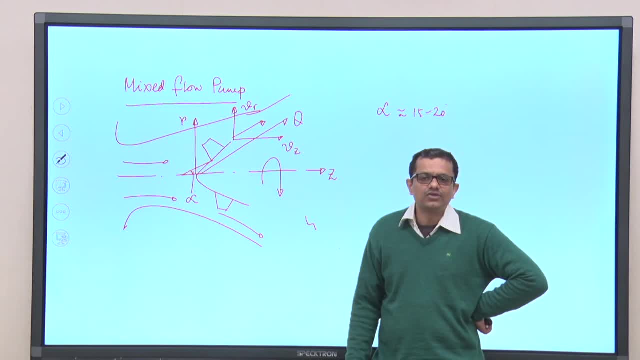 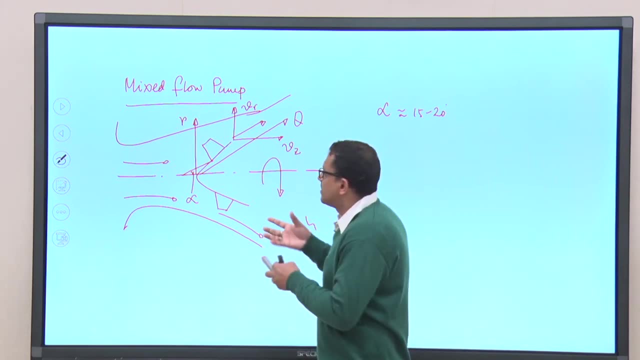 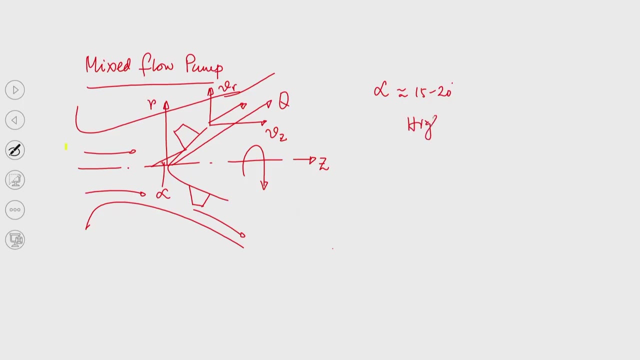 in a condenser, we need to supply cooling water. So in a condenser, cooling water due to is pump, which are the mixed flow pump. So basically, these mixed flow pumps are used where we need, where we need high discharge, and moderate to moderate head, I will say moderate head, moderate head. 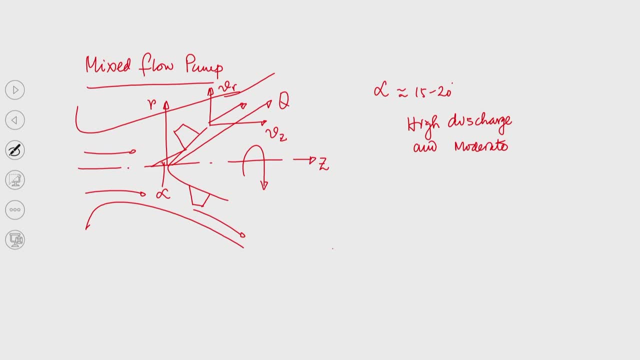 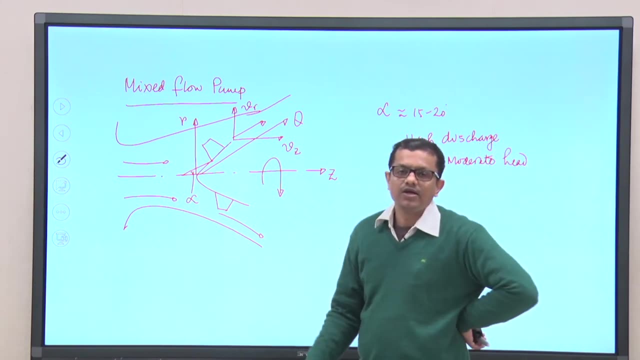 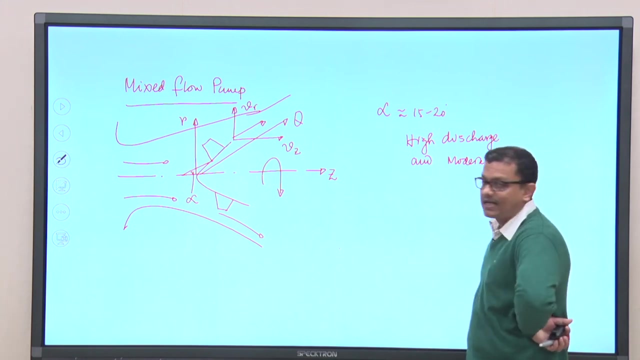 So it is moderate head right. So the mixed flow pumps are used to supply condenser cooling water supply. I mean there is to supply condenser cooling, you know cooling water, and this pumps are used where we need at least high discharge against moderate head. special feature of this pump is that the impeller 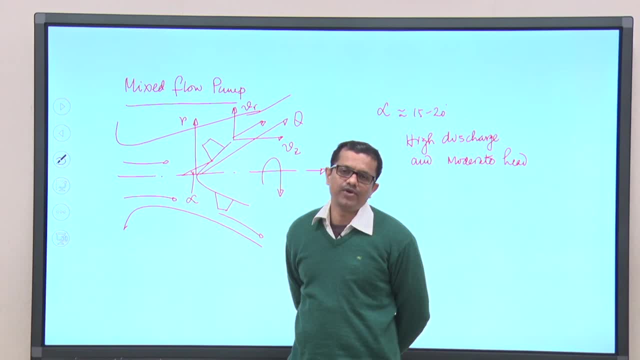 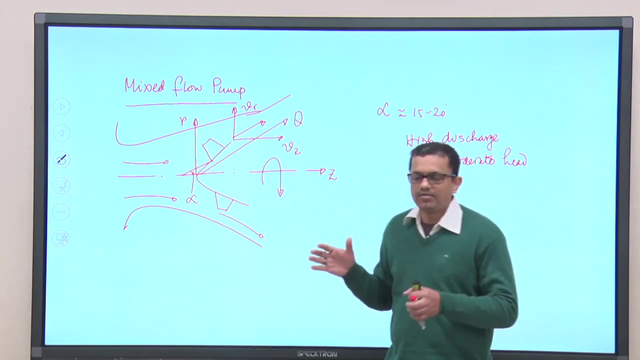 diameter is of the order of 1.5 to 2 diameter and it consumes huge power for its operation. So this pumps are not typically used. the most important applications, most important application of this pump is condenser cooling water duties pump. So the because this pumps diameter is very, very big it it it occupies very large space. 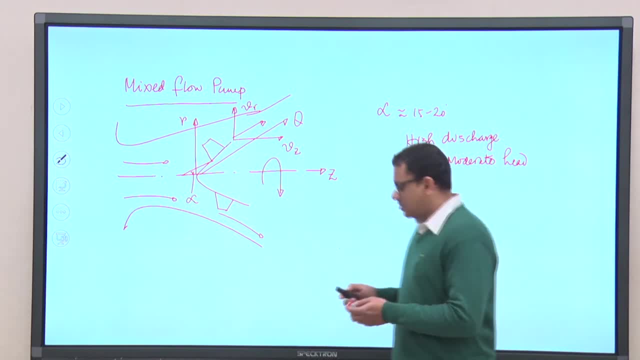 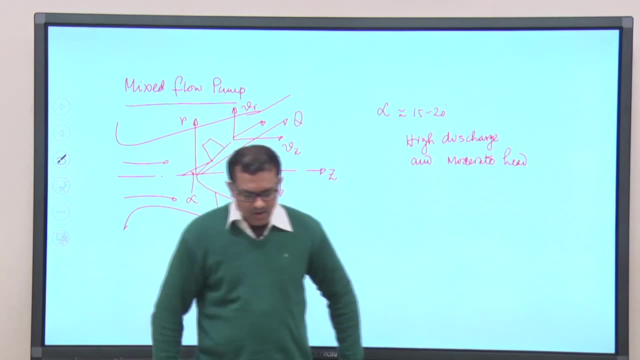 so the power consumption is very high. So we have discuss about the classification of, you know, hydraulic machines. we have also discuss about the basis on which we can classify hydraulic machines into different groups. And then, finally, we have seen that the roto dynamic pump, which can be classified based 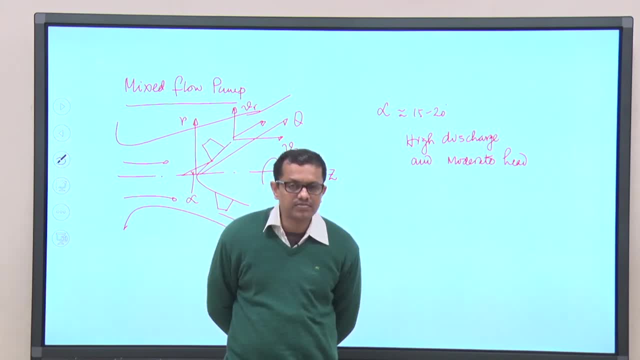 on the direction of fluid flow And into three different groups, and we have discussed all these types, that is, radial flow, axial flow and mixed flow, and we also have identified their applications. I mean I mean the most important applications where these types of pumps may fit. you know applicability. 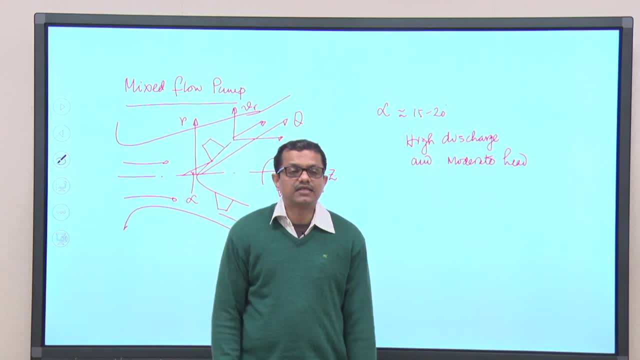 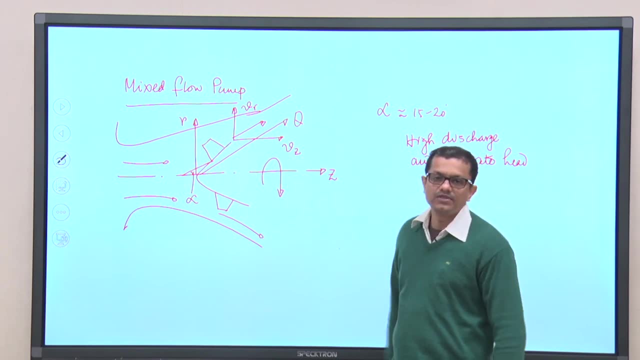 and also we have discuss about Dependence of force, that is, whether it is whether centrifugal force is there for the, you know, increase of the velocity and pressure in of by a bio pump, or it is not the centrifugal force. So finally, I would like to discuss that we have seen that, whether it is axial flow, 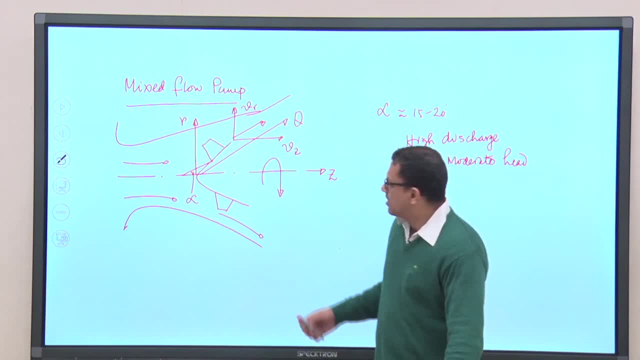 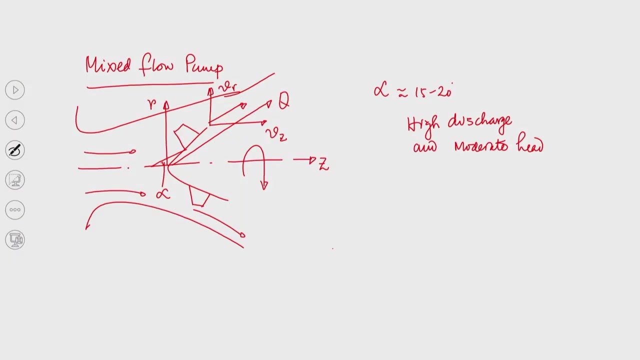 radial flow or mixed flow In when fluid flow is there, That means fluid flow, that the flow dynamics inside the pump is highly three dimensional, because we have seen that if I try to draw one impeller again, right. 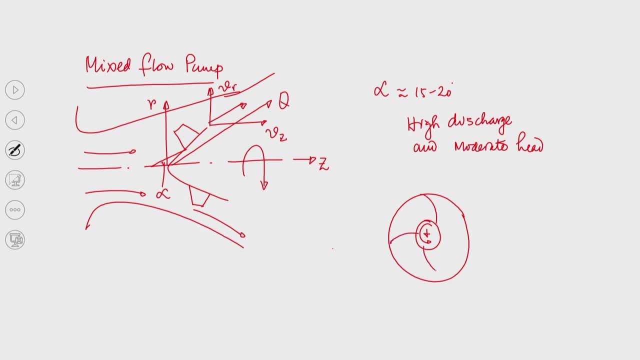 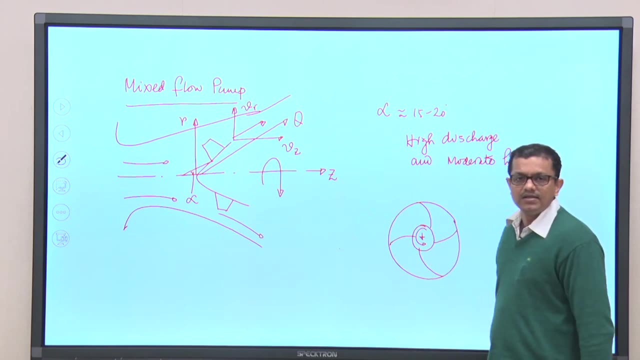 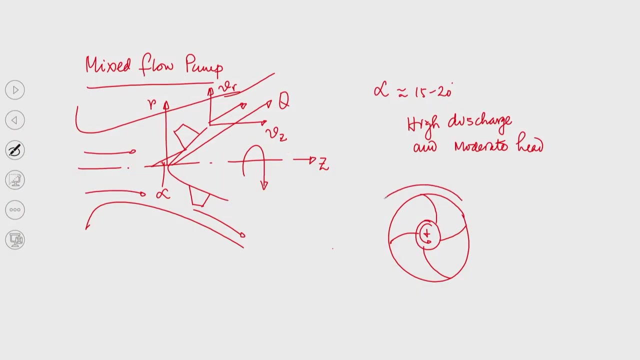 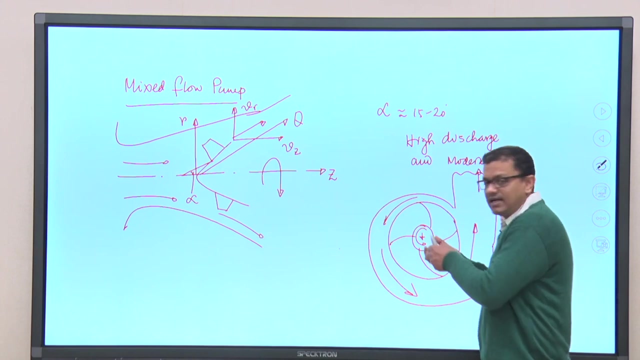 So this is the typical, you know, schematic of a radial flow pump, if the inlet is perpendicular. 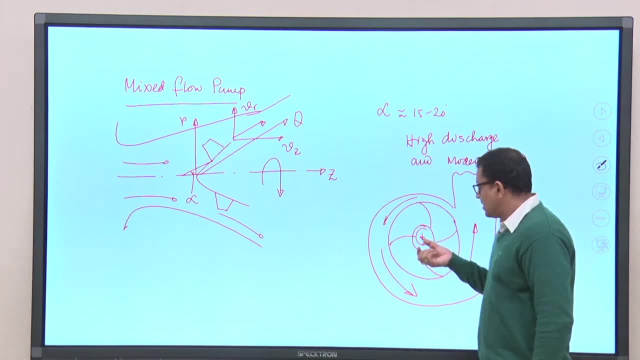 to the board plane of the board and if we allow that means if the intake of water is in this direction and then work is done on the fluid, by virtue of the rotational effect of the impeller and liquid will move in this direction, it will be guided by another part. 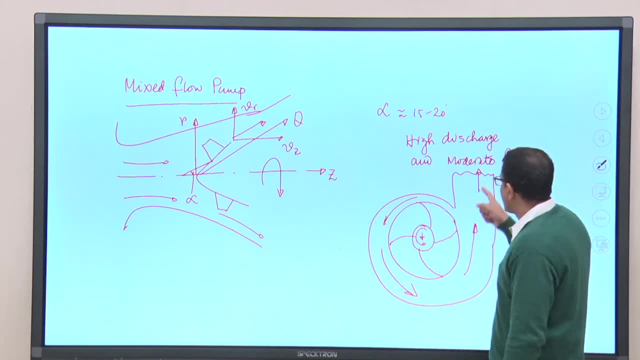 which is known as pump casing. that we will discuss later and eventually we will have liquid which is coming out from the pump having high pressure and velocity. So what we can, what I would like to discuss over here, is that the flow fill inside the pump impeller is highly three dimensional.